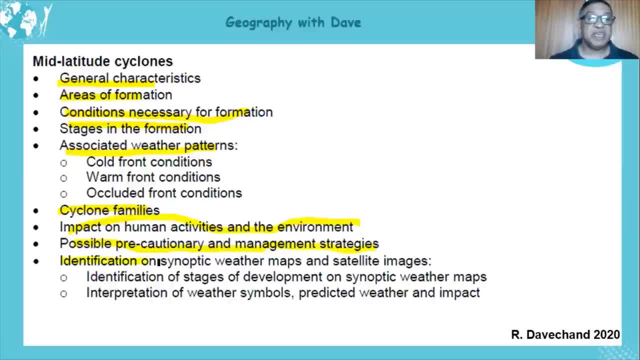 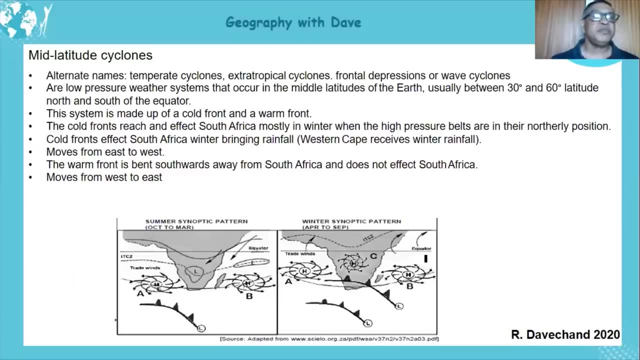 and management strategies, identification on a synoptic map, satellite images- okay, We look at various of these things, okay, and we'll go ahead and we'll simplify it The thing for you. alright. Now let's start off with the basics of our mid-latitude cyclone. 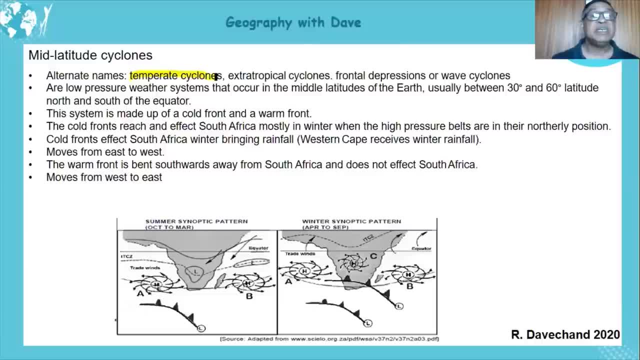 First of all, we need to know that there's alternate names: temperate cyclone, extra tropical cyclone, frontal depression, wave cyclone- So these are various names that can be used for calling or naming mid-latitude cyclones. 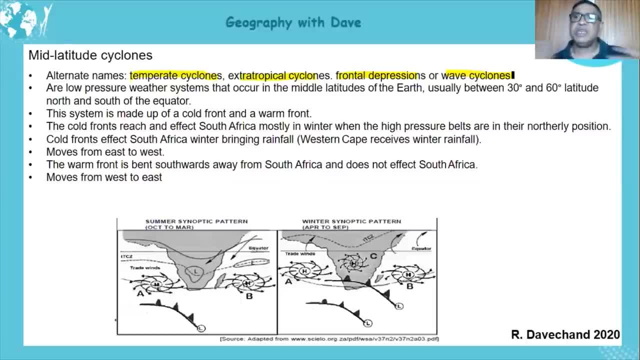 But the common one we find is always used in exams, et cetera, is the term mid-latitude cyclones. Now, we need to know that it is a low pressure system, alright, and it occurs in the middle latitudes of the earth, usually around 30 to 60 degrees Celsius. Okay, when? 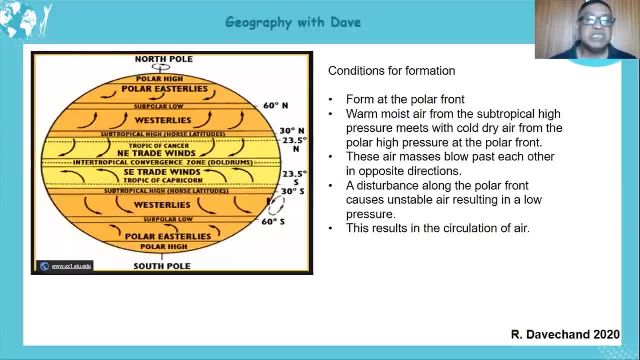 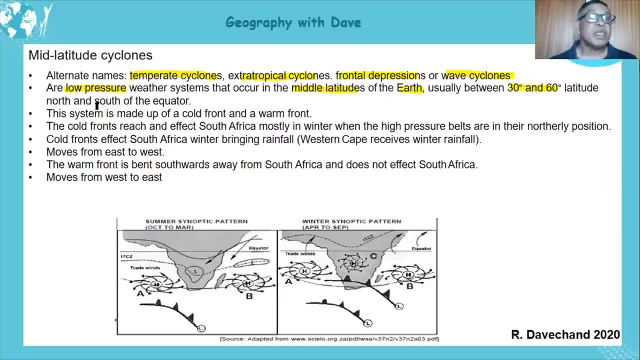 we look at it here, In this region, it occurs- okay. Now it occurs north and south of the equator, on both sides right of the equator. you get this Two distinct characteristics. it's made up of a cold front and a warm front. Don't mix, we find. sometimes talk about the eye, et cetera. 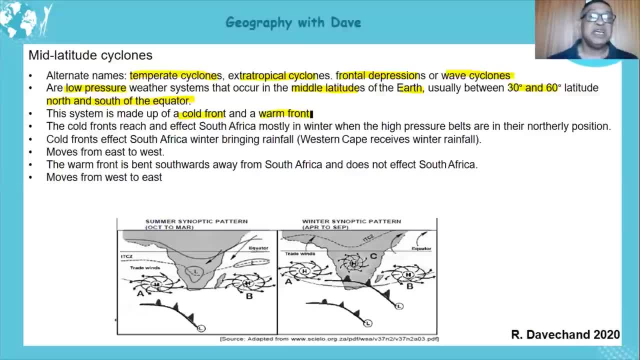 This. that's the tropical cyclone. Here we have a cold front and a warm front. Cold fronts reach and affect South Africa mostly in winter. Sometimes they're getting them coming through in late summer, et cetera, when high pressure belts are in their northerly position. 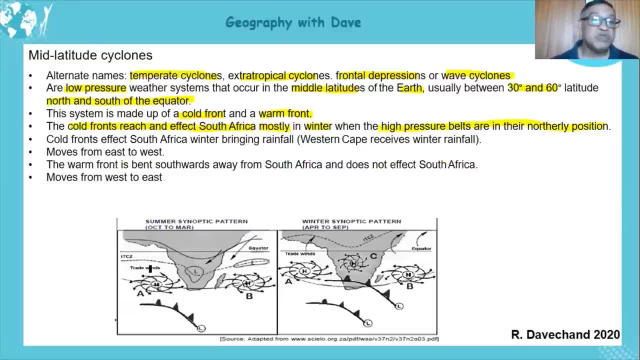 Now I'm going to show you here. Remember your teachers would have told you about the ITCZ. When it's summer in the north, it's called ITCZ. When it's summer in the south, it's called ITCZ. 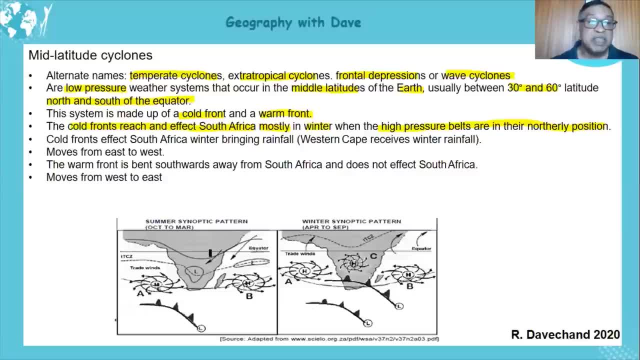 Okay, When it's winter in the southern hemisphere, remember, the ITCZ moves southwards, All right. And when it's winter in the southern hemisphere, the ITCZ is found in the northern hemisphere, and the ITCZ into tropical convergence zone is a low pressure area. 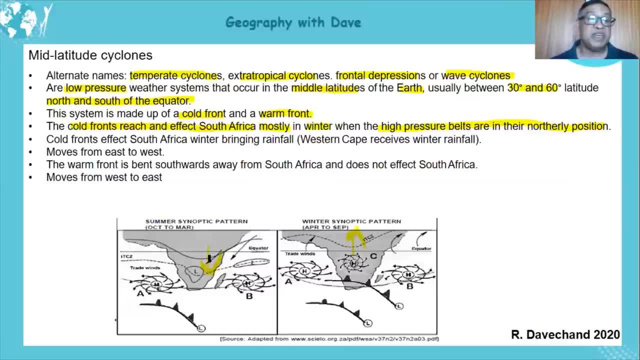 So what happens when it's in the southern hemisphere, the ITCZ, the high pressures, don't move up, Do you understand? So they stay in their southerly position because it moves from high pressure to low pressure, You understand? And when they it's winter in the southern hemisphere, then the ITCZ is obviously in. 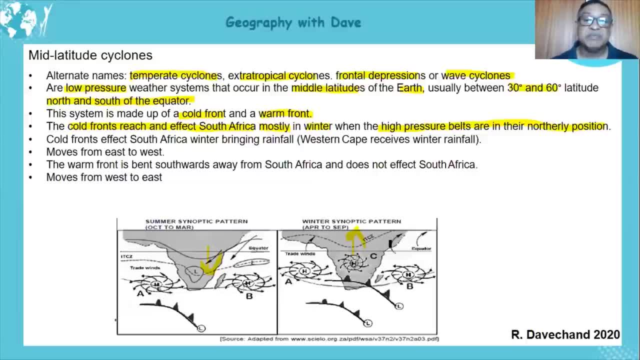 the northern hemisphere and the high pressure systems will move towards this low pressure system and there'll be in a northerly position. And this explains it, because if these high pressure systems are in their southerly position, especially in the northern hemisphere, they'll 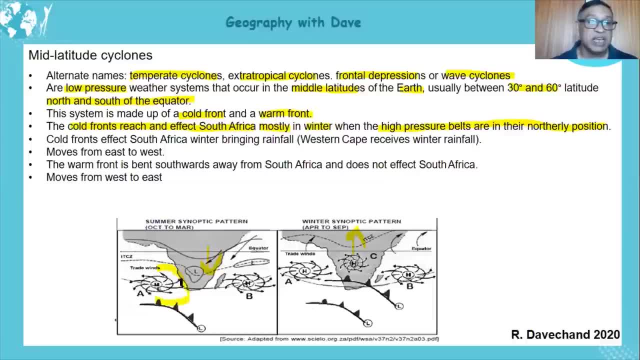 move up, Okay, Especially the South Atlantic high. it's going to ridge and block the cold front from coming in, Okay. But if it's in its northerly positions it's moving north. You understand What happens now. It allows the cold front to come in and effect the country. 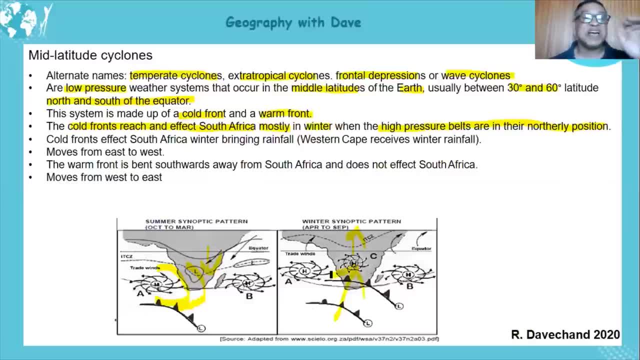 Okay, So that is why you have cold fronts effecting the country, mostly in winter, All right, And they bring in cold fronts, effect South Africa winter in winter, bringing rainfall, like in the Western Cape you'll find they receive winter rainfall because of the Mediterranean. 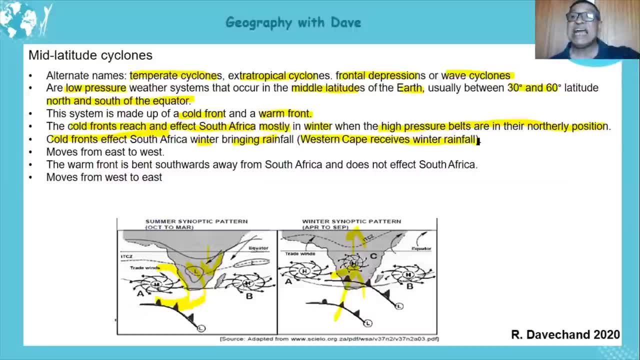 climate, obviously, and because of the cold fronts coming in and uplifting the warm air, You understand, Creating condensation, cloud cover, And the rainfall occurs. Okay, And there, whoa, a gremlin creeped in here, All right, 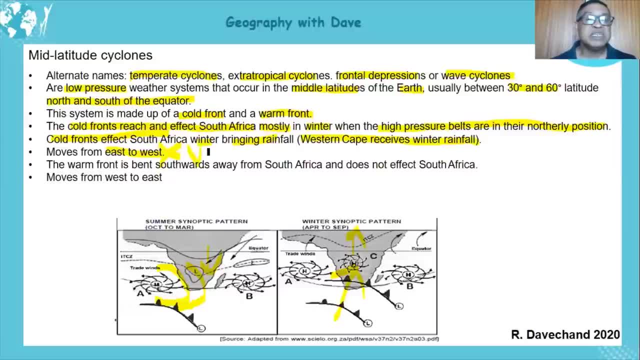 Wrong. It moves from west to east. Okay, North east to west. I apologize for that. From west to east, All right. So it moves from here West to south, west towards east. sometimes it's also known as southwest to northeast, but the general direction 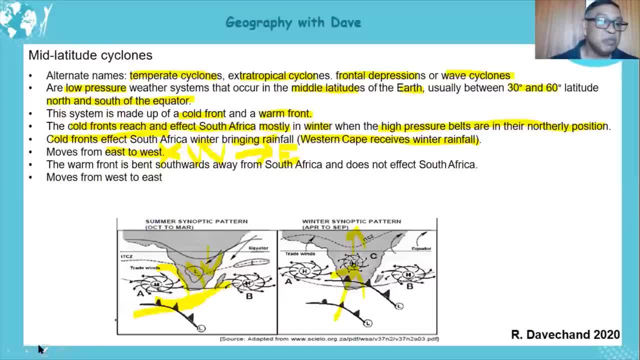 is from west to east, so i'm going to put a red line here. no, my apologies, i'm now getting mixed up. okay, so it moves from west to east. we'll talk a little bit more about it. all, right, as we go through the formation and we find that what actually happens here, just in a brief, and i 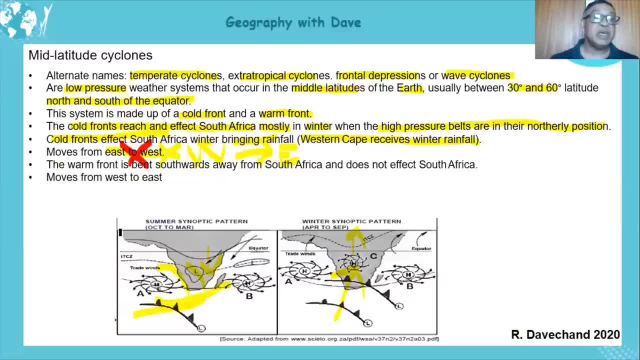 know it's not, uh, really making sense at the moment. when i say the warm front bends southwards, away from the cold front, you understand in a way. so therefore it does not affect south africa. okay, i'll go into a little bit more detail of this later on. 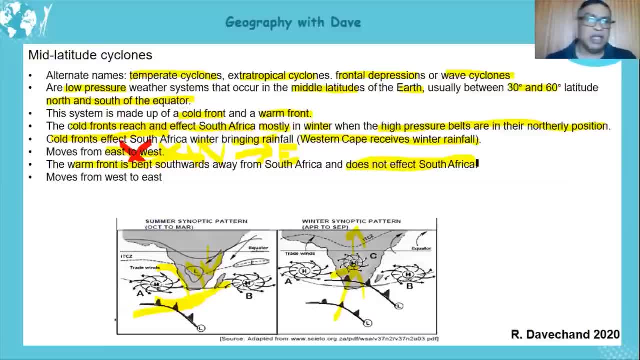 okay, so we basically can sum up from here that the cold front affects our country, south africa, and not the warm front. okay, and i've got it right here. it moves from west to east. my apologies, learners, it's my gray hair down here that's actually made twice and 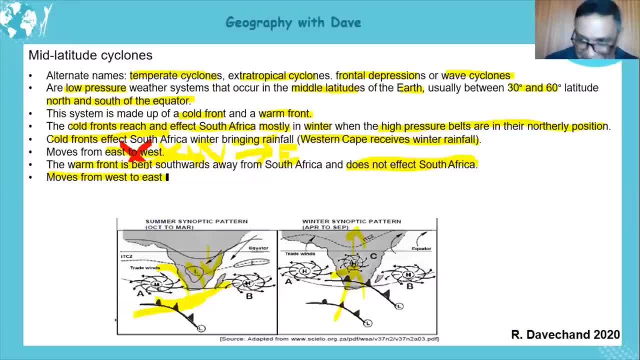 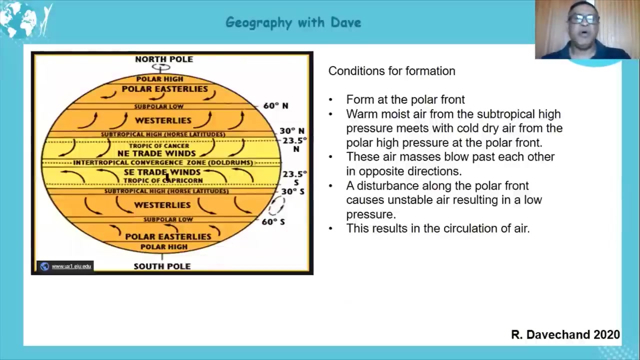 put in the tropical cyclone movements. so i do apologize for that. okay, all right so, but it's good actually, on one hand, that i showed you the difference already. i'm trying to make excuses. okay, so it moves from west to east right now. how does it form? okay, how does it form? 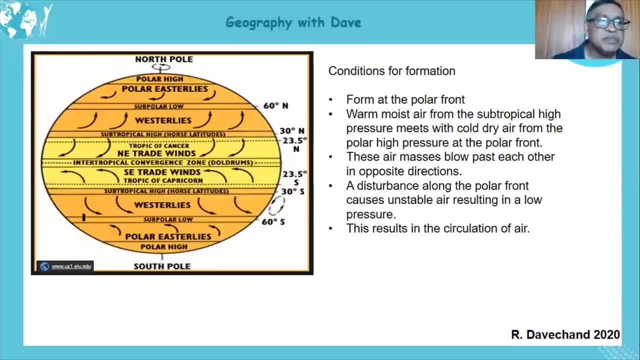 now, if we take this area here, all right, the sub polar low- we've learned along this area- is the polar front. okay, the polar front. it's not totally stationary, although on many occasions it's considered stationary. right now that's the polar front. it forms at the polar front. 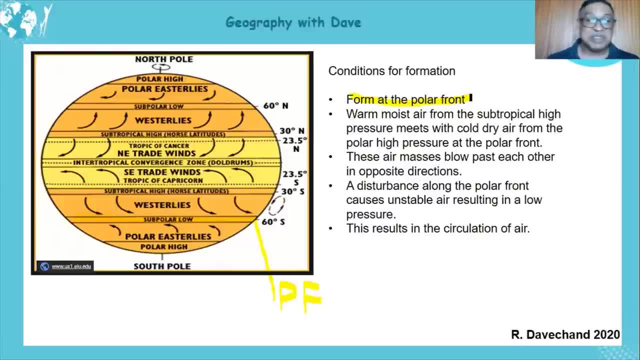 it starts to fall. okay, that's what we must remember. now, what happens here? warm moist air from the subtropical high. there we have it here. the warm moist нашей is coming in all right towards the subpolar low, all right, which actually has warm moist air pressure belt. it meets with the 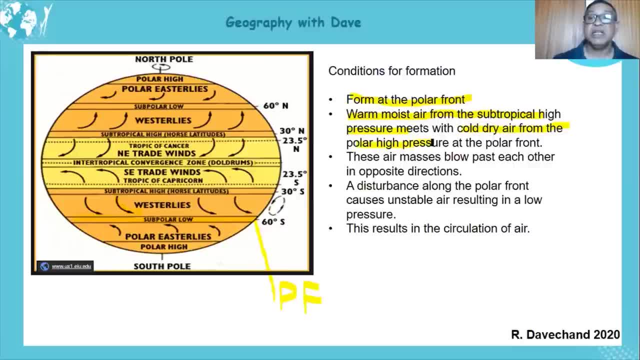 cold, dry polar high pressure. a all right at the polar front. can you see? there's the cold, dry polar air moving in here. obviously it's being deflected right due to the rotation of the earth and coriolis force. so what do we have here now? warm, moist air from the subtropical high. 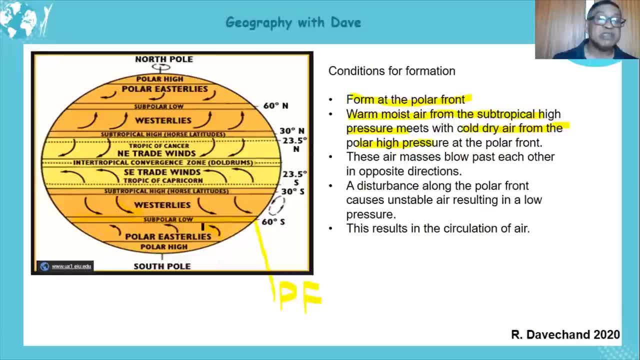 cell and cold, dry air from the polar cell. they meet on both sides of the polar front, all right. these masses blow past each other in opposite directions. so if i look at this, it's flowing this way, all right. and if i look at this, it's flowing in the other direction. 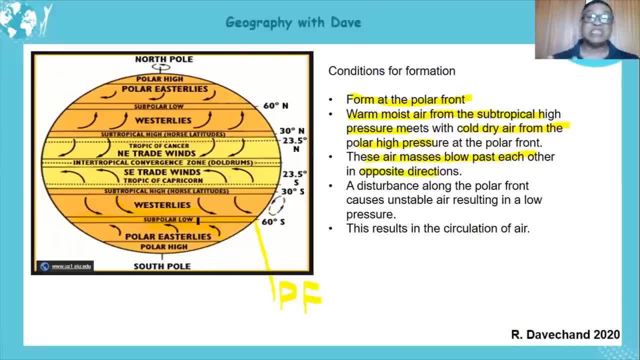 so we have two an opposite directions, on both sides of the polar front. then a disturbance is created along the polar front which causes unstable air. so what happens along the polar front? there's a disturbance, a bend, you understand? oh, i can make a bend like that, okay. so what happens? there's the cold. 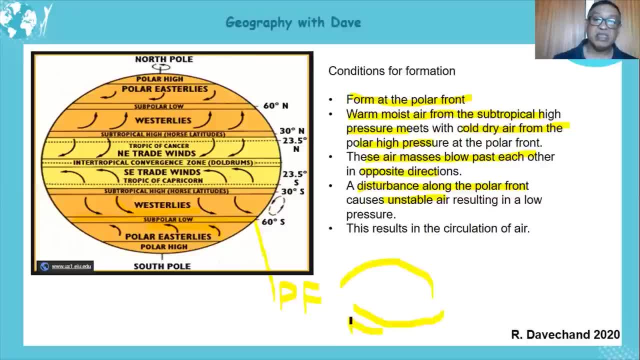 air moving here, all right, as shown down here. and there's the warm air moving this way, can you see it? it moves southwards. this disturbance, this bend- all right- will then cause the cold air to come in here and force some of the warm air up here. and if it does that, 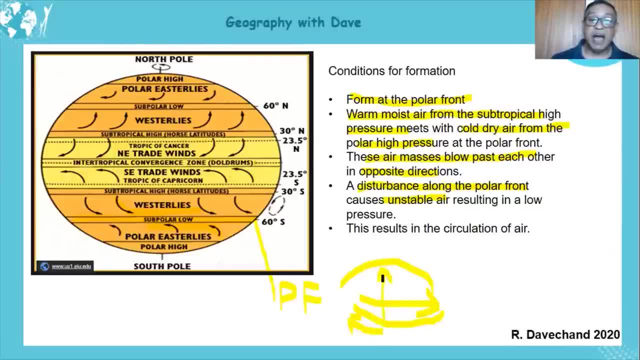 you understand, unstable air is moving up, all right. this creates a low pressure around that point, because once air is uplifted, you will find a low pressure being created. that is your start now. obviously, when this starts happening, it results in a circulation of air. obviously you can see the cold air on. 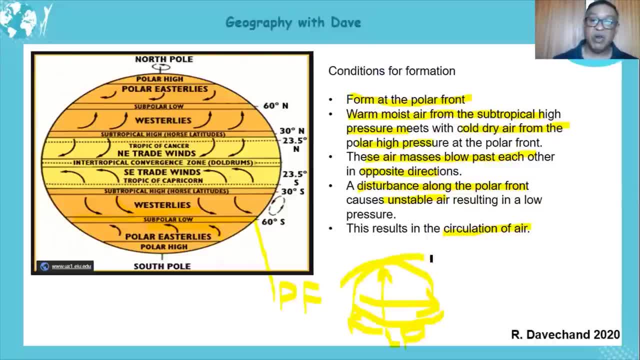 this side moving warmer that side, and you can see all the air that's going in a clockwise direction. okay, because the warm air is pushed further south and the cold air is moving more northwards. okay, and that starts the circulation. i want to draw something here. okay, 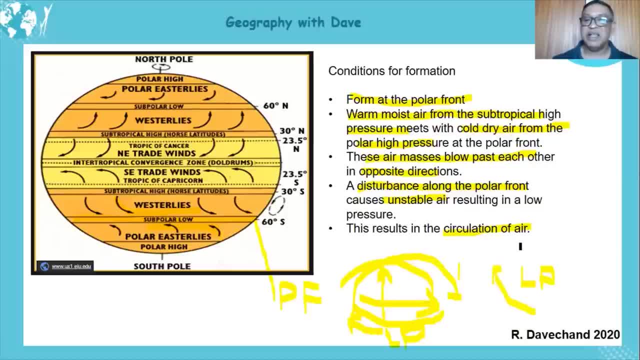 there's it moving that way and that way. now the circulation of air has started in that area and then you start getting your middle attitude cyclone starting to form. okay, we just got a rough idea there. that is why we are to bring in our grade 11 work to look at it. 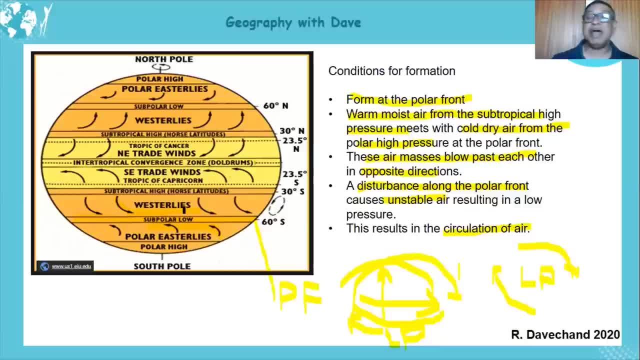 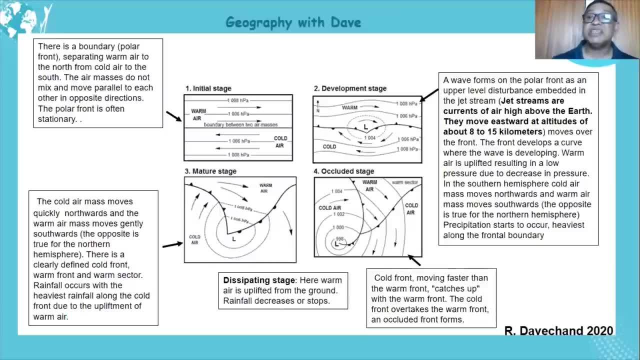 and this obviously is in the westerly belt. okay, you've done that in grade 11.. okay, let's go further now. let's look at the stages. okay, now i know there's a debate. we call it the initial stage and we always debate this. nothing has really happened. 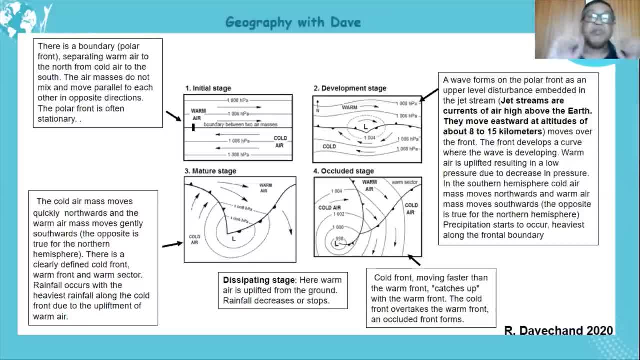 this is how the flow happens at the polar front, but we're not going to look at it that way. we're going to call it the first stage, all right now. you already saw that the warm air from the subtropical high coming in the cold polar air. we're not showing the 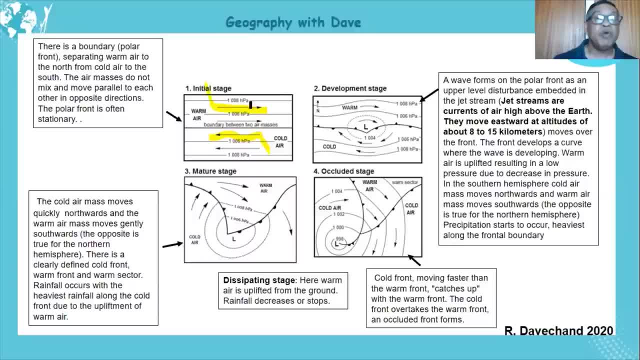 deflection here, but that's how it comes in. they're flowing in opposite directions, all right. so we say there is a boundary, the polar front, separating the warm air to the north- okay, that's in the north- from the cold air to the south. that's your polar air coming in. the air masses do not mix. they're on both sides of the polar front. 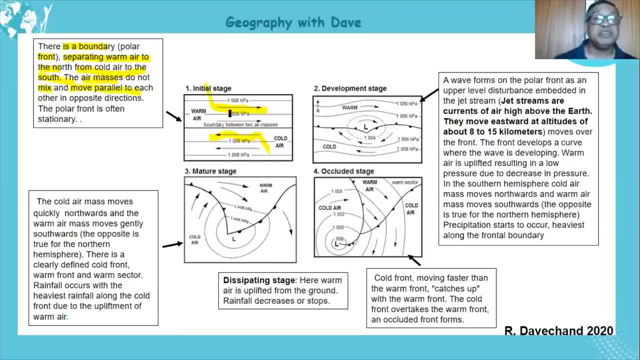 all right, and air moves parallel to each other. can you see this one in this direction, as shown by the arrow, and this one in this direction? the cold, dry air, all right, from the polar. so they move more or less parallel to each other in opposite directions. okay, can you see it again? opposite directions. 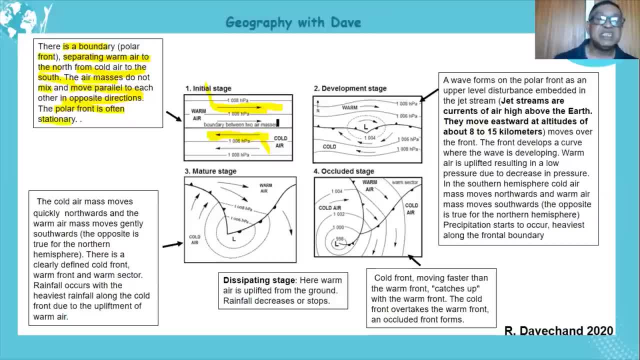 the polar front is often stationary. it stays in one, not always all right. the polar front can move. it's not always at 60 degrees so it can move, but on many occasions it can be considered stationary, but overall is not always stationary. we must remember that right now. what's going to happen? all right? 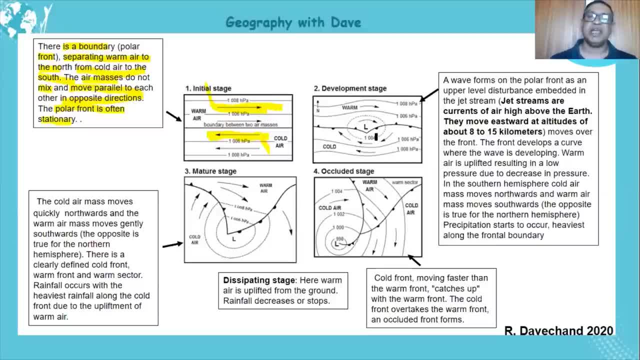 this is when the cyclone really starts to form the middle attitude cyclone and we say a wave forms on the polar front. all right, there's the wave here. can you see it? all right, it can be surface obstructions also, but one of the big things that actually cause this wave, all right, 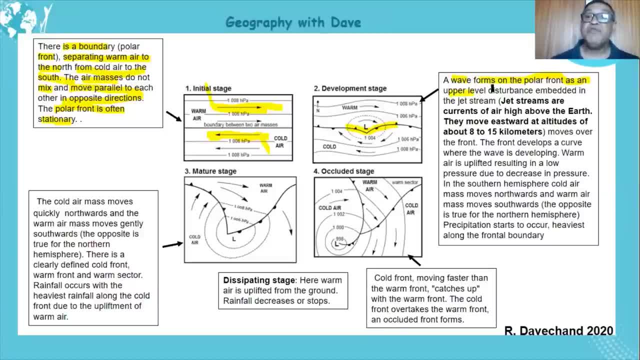 in the upper level, sorry. a wave forms in the polar front as an upper level disturbance embedded in the jet streams. so upper air disturbance happens here, all right, can be surface also, but the upper level, and now this jet stream will cause a disturbance, all right. so what is a jet stream? all right, jet streams are currents of high above the earth. 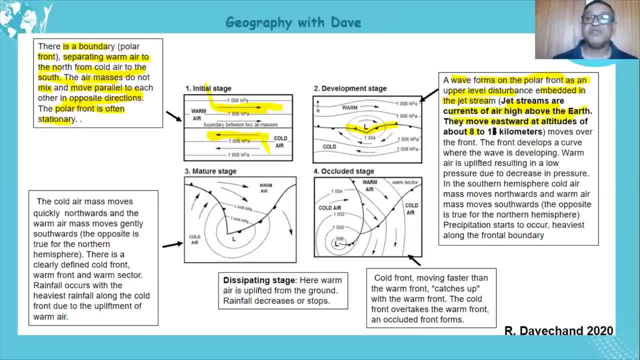 they are found there. they move eastwards at altitudes of 8 to 15 kilometers. so there it's moving eastwards. all right, these jet streams, and as they move, all right, they create a disturbance. yeah, moves over the front, over the polar front. can you see it moving there? all right, and the front. 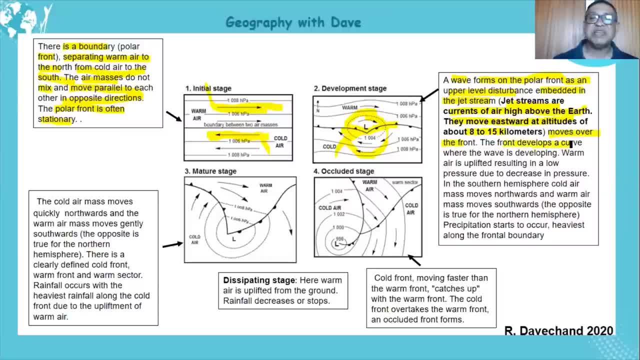 develops a curve, all right. it moves eastwards, right, develops a curve- okay, where the wave is developing, the bend and the wave is developing, of course, the warm air is now uplifted because of the curve. the cold air is moving in northwards, southwards and warmer gets uplifted, all right. 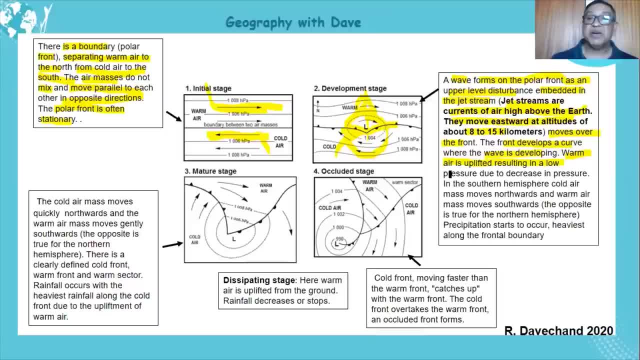 pressure decreases here. all right, pressure. you decrease in pressure, all right, and you can see clearly here, because the air is rising, so the pressure is decreasing. in the southern hemisphere cold air moves northwards. can you see? the cold air now is moving this way because the disturbance has been played. the wave is there, it's moving northwards. 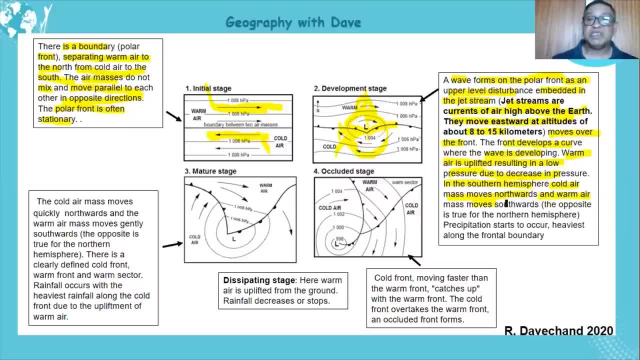 and the warm air moves southwards, as i showed you earlier. i'm repeating myself, but it's good that we do that, because it's pushed like that, all right. of course, the opposite is true for the northern hemisphere, in the sense that, uh, it's facing that way, all right. 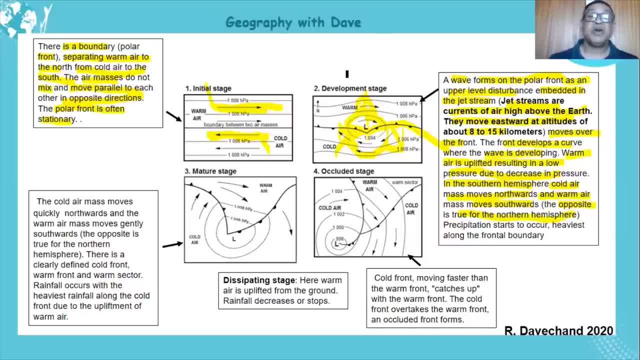 so we have a situation where the cold front- if it's sitting like that and we have a disturbance, then the cold front will move southwards, okay, southwards right. precipitation starts to occur, and heaviest along the frontal boundary, along this area. so we already start having precipitation. 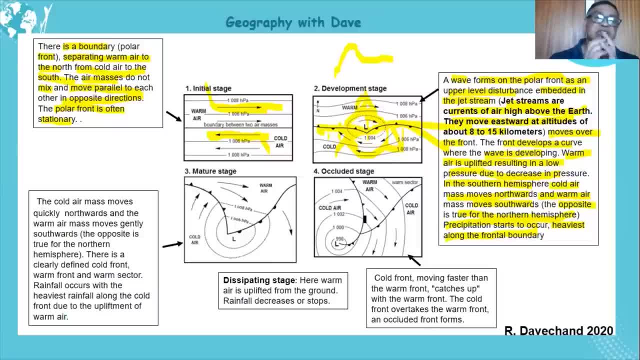 in this area. okay, air, all right. so that's the development. then we reach the mature stage now. first of all, you see the wave there and you see two distinct fronts here. now they are completely, uh, away from each other. all right, can you still see the northward movement here and the eastward movement of that? 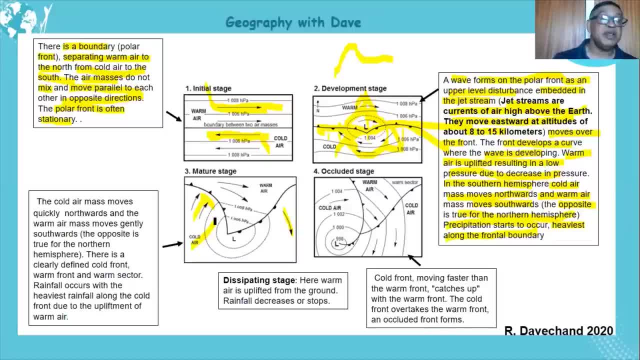 due to the disturbance when the jet streams came in, all right. so it's clear, it's distinct. we have two clear, distinct fronts: cold front, one front, and that's how you know it's. in the mature stage they do meet at the apex, at the low pressure, so cold air moves quickly northwards. 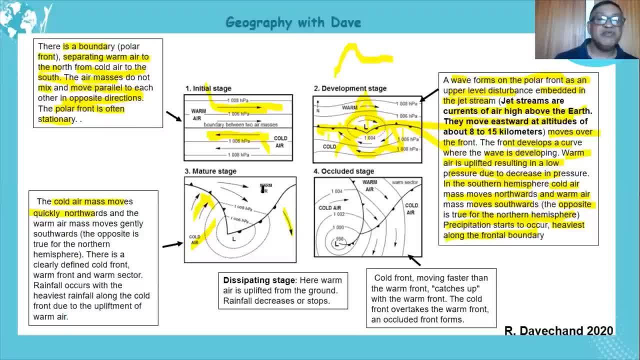 there's it, moving rapidly. now, all right, forcing the warm front southwards. and the warm front moves gently, all right, because it's also not, you must remember, this pressure gradient is steeper at the cold front because it's cold dense, you understand. so it moves, that steeper gradient. 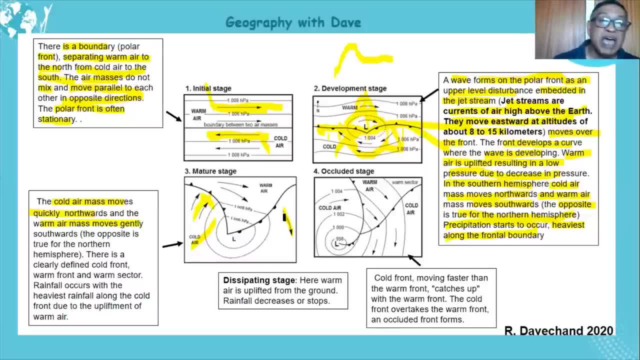 you understand, there's more movement and of course it's warmer at the warm front, so the gradient is more gentle, a slower movement, all right. southwards, okay, obviously it's the opposite. in the northern hemisphere, okay, there is a clearly defined cold front and warm front and warm sector. so there you can see clear. there's no mixing like this. 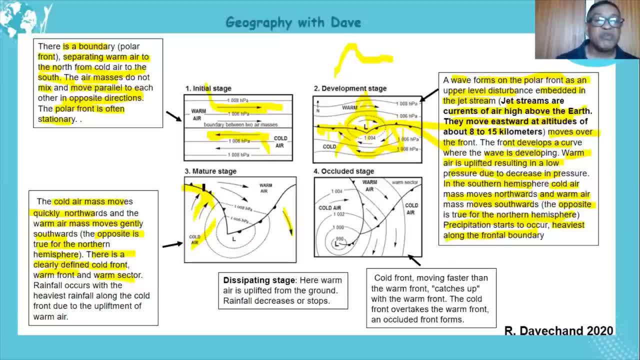 warm, cold, whatever. it's clear, just a cold front- i call them the thorns, you can see it there- and a clear warm front. this is the mature stage, i call them the semicircles. and in between, the warm sector, clearly show, all right, clearly show, okay, rainfall occurs. 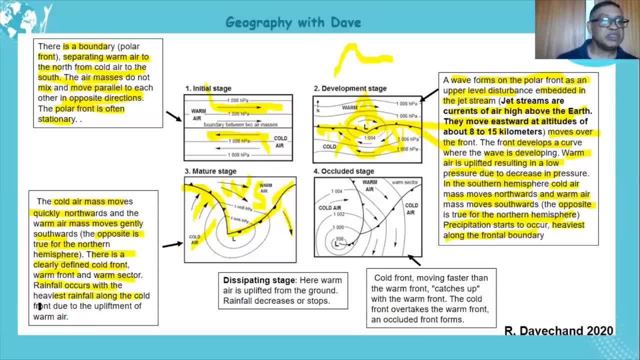 with the heaviest rainfall along the cold front. remember the cold front has got a steep pressure gradient. i'll do that in a little more detail. we'll look at the cross section also- steep pressure gradient. you understand, so it's gonna. if it's a steep pressure gradient, watch my hands there's. 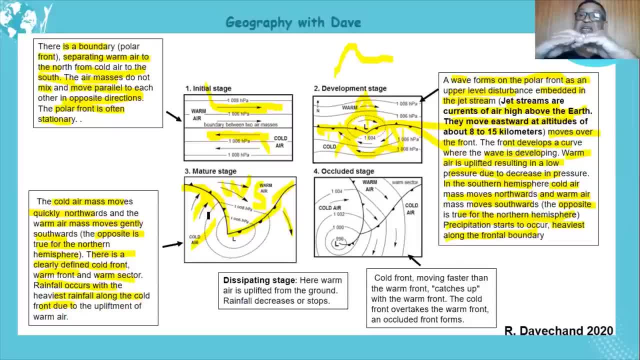 the warmer here it comes in and lifts. there's rapid upliftment all right of the cold front. you get a consistent rainfall and it's heavier. you see too'll. you'll get rain at the warm front, but it'll be less. you get consistent rainfall. so you see the rapid upliftment, and this is why. 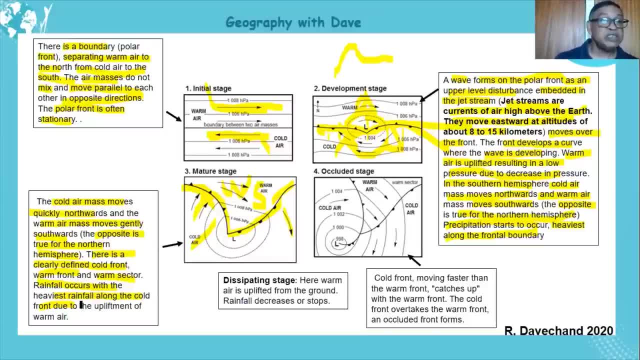 you'll find that it's the warmer air in front because of this steam pressure gradient and pushes it up. that is why you'll find cumulonimbus clouds etc. forming here, but we'll talk about that later. all right, so heaviest rainfall along the cold front due to the upliftment. and i would like to say 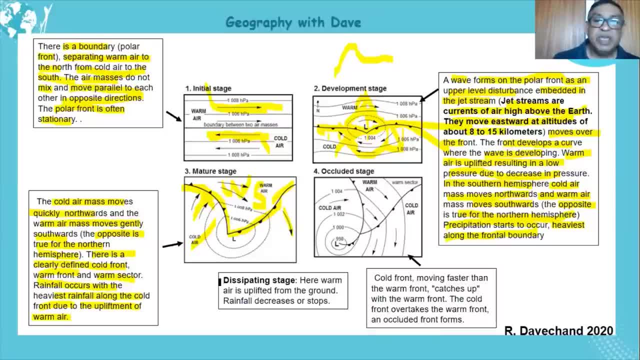 in rainfalls, etc. then we have the next stage, which is the occluded stage. now what happens here, remember, the cold front is moving faster than the warm front. you know why? now it's deeper pressure gradient and whatever. so what happens is the cold front moving faster than the warm front. 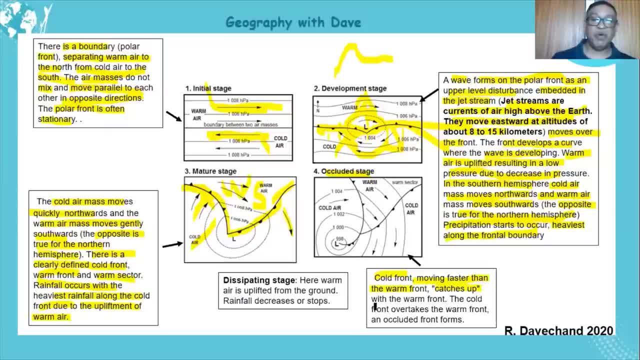 and then the warm front catches up with the warm front, can you see it here? catches up with the warm front. you understand, can you see them here? clearly indicated, all right. and then the cold front overtakes the warm front, forming an occluded front. you understand generally the term occlusion. 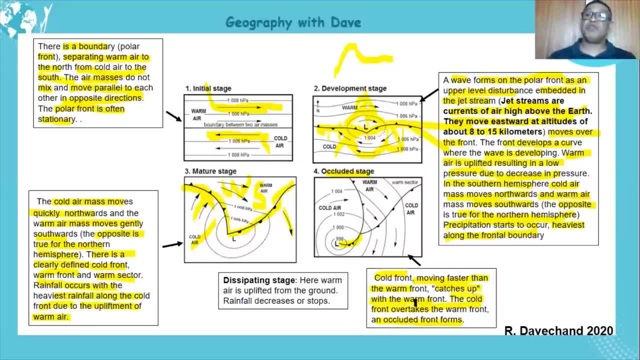 warming, you understand. so in all types of occlusions, you must remember: warm air is uplifted, you understand, or the warmer air is uplifted. sometimes you get a mistake. we think warm, we talk 20 degrees or whatever, let's put it. the warmer air is uplifted. and then, of course, last one, and I don't have a diagram for it: 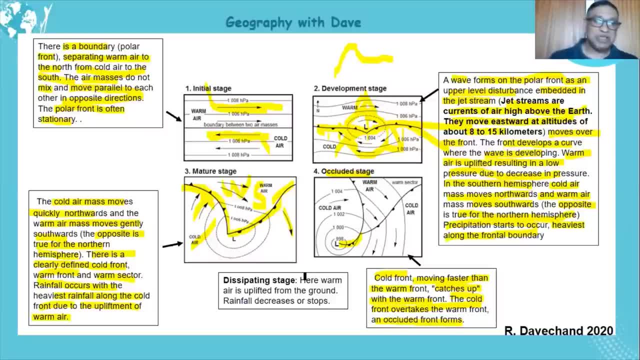 because now the cyclone doesn't exist anymore. so we have the dissipating stage. yeah, the warm air, all the warm air, is uplifted from the ground. so the warm air is gone. what stays at the ground now it's the cold air. of course, pressure will. 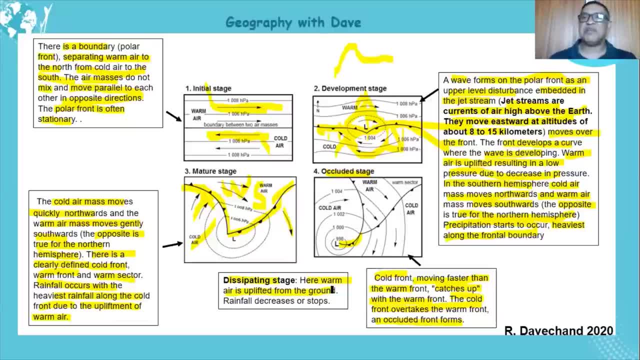 increase, you understand, and there's no low pressure now. okay, because all the warm air has been pushed up. and then what happens is the cyclone dissipates, finished and, of course, rain fall will cease because there's no more warm air rising. okay, and therefore the cyclone. 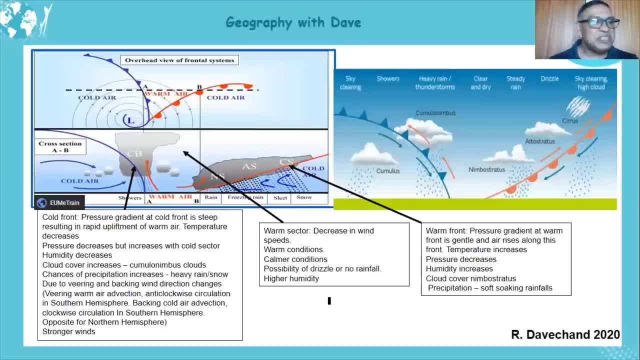 clone is gone. okay, now let's look at the cross-section of this. okay, I showed you a view of how it look. cold front, all right. warm front, all right. this is the occlusion. but I'm showing you here: cold front, warm front. okay, it works like that. 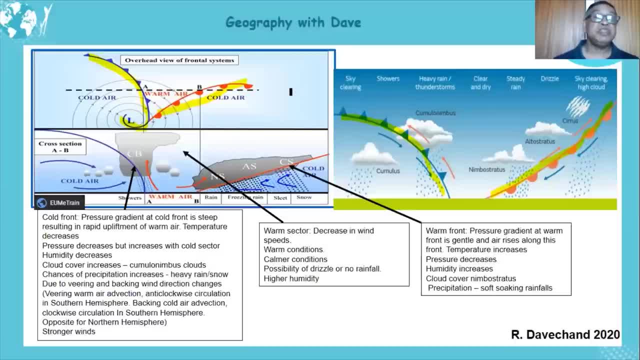 and depending where you're talking about, why I put these two diagrams. if you get a cross-section last, you draw a cross-section and you look at this and you see occlusion, you understand, also must run included front watch, where the examiner is asking you to draw the cross-section. and if you look here, he's. 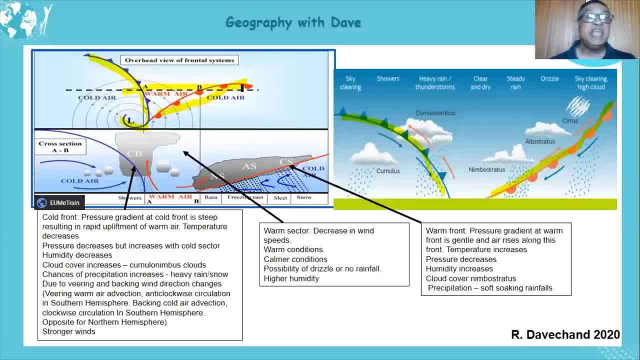 asking you, for she's asking you from A to B Easter you the occlusion at A to B? no, so watch, be careful about that. if it was down, here was a different story. there's an occlusion, but it's A to B. there's no occlusion occurring there. 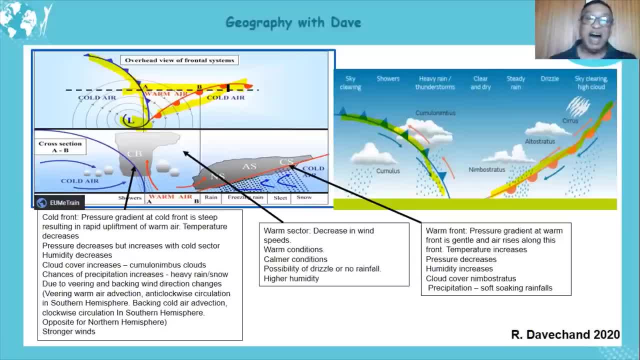 the warm front, the cold front and the warm front are separated. now, learners, please, you guys lose marks. you do everything correctly. when an examiner is asking you to draw the cross-section, all right, you draw the cross-section and you here the same thing from A to B. so you put a cross-section here, like I said. that's. 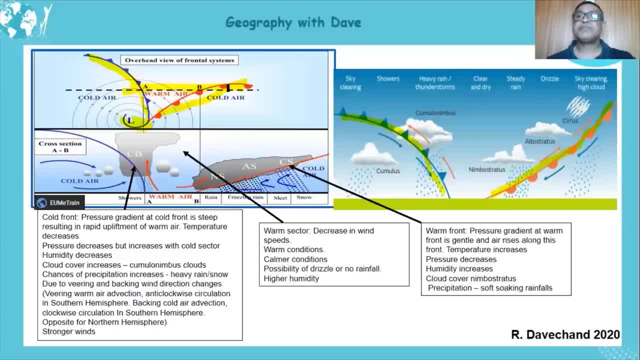 19 a♥, 12, 13, 14, 15, 17, 18, 17, 18, 19, 19, 10 And blue. if you want to, you can do so In terms of a cross-section. you just have a pen in front of you. 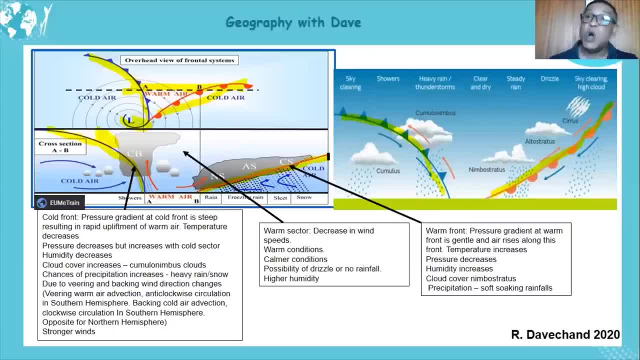 It doesn't matter about the colors, Okay. so please note that. Okay, that it's just lines representing them, not those thorns, as I call them, or semicircles. It's incorrect. You get no marks for that. 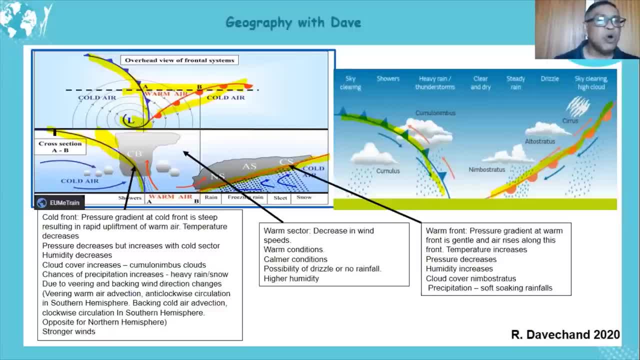 Okay, we've got that clear. See, let's start off with this cold front. All right, we can see, down there there's this cold front. Okay, so cold front Pressure gradient at the cold front is steep, You can see it. 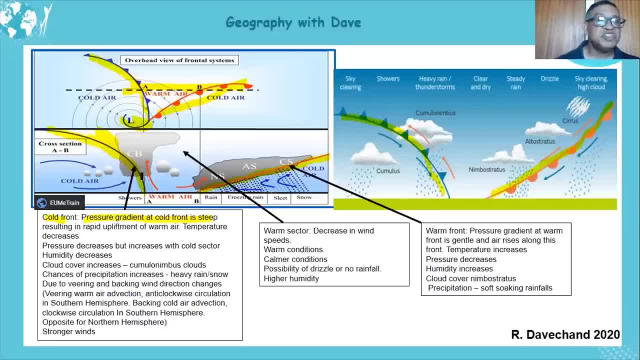 It's steep because of the cold air, You understand. it's steep, All right, resulting in rapid uplift of warm air. All right. when the steep gradient comes in like a bulldozer, all right, and forces this warm air up. 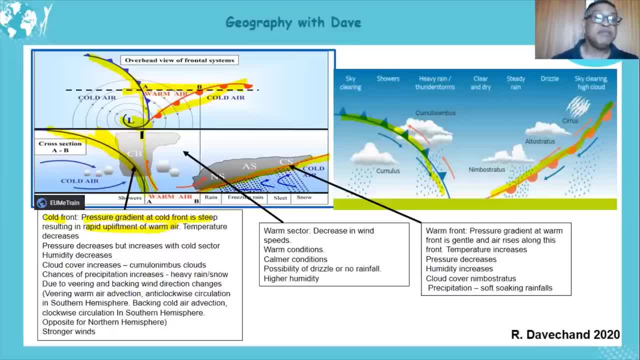 So there's rapid uplift, And it is rapid upliftment, It goes to a higher extent And as it cools, it's going to form a cloud of vertical extent- Cumulonimbus clouds, Can you see? That is why you get your big clouds in those areas. 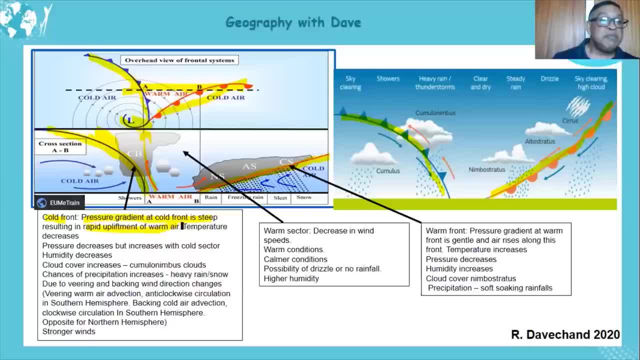 All right, obviously right. the temperature decreases because it's a cold front coming in. The pressure decreases because, if the air is uplifted at this point, there's less air here- am I right? Resulting in a low pressure. All right? 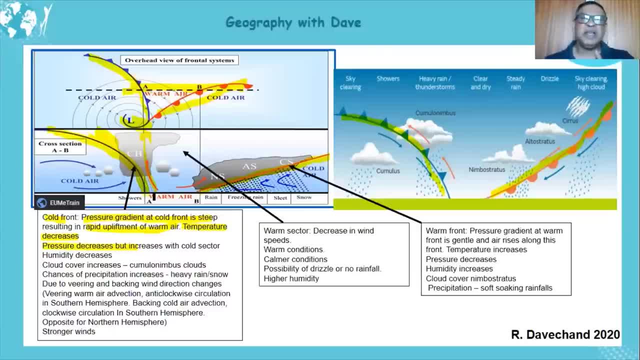 All right, Resulting in a low pressure. All right, Resulting in a low pressure. That's how you read it. all right, I know many resources you have just says pressure decreases, But why? Because the air is getting uplifted. 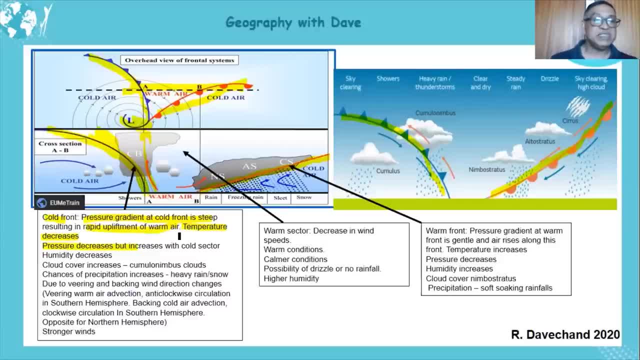 Therefore, less air here. pressure decreases With the cold sector, all right, but increases with the cold sector As this air is warmed up, then the cold sector comes in. There's more air near the surface, Less air, Less air. 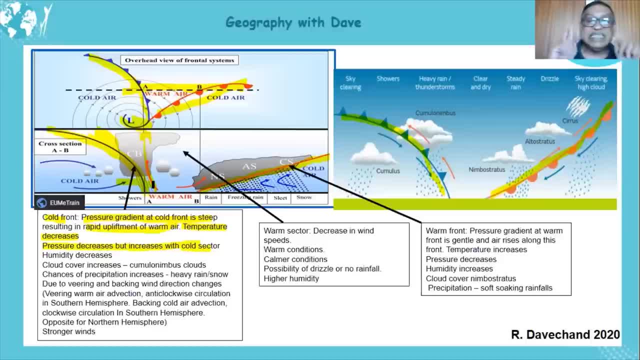 And the air is rising here, Obviously the pressure will decrease or increase, rather, because now it's subsiding, So the pressure increases, Humidity decreases because of this air coming in here, The cold front, You understand, And the cold sector. 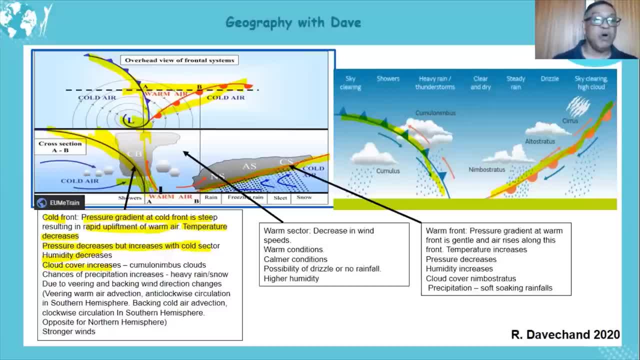 All right, Cloud cover increases because all the moisture is being forced up. You understand, there's condensation and the cumulonimbus cloud is forming, So cloud cover increases, increases and you get this cumulonimbus clouds because a is rapidly uplifted, so we get this cloud. 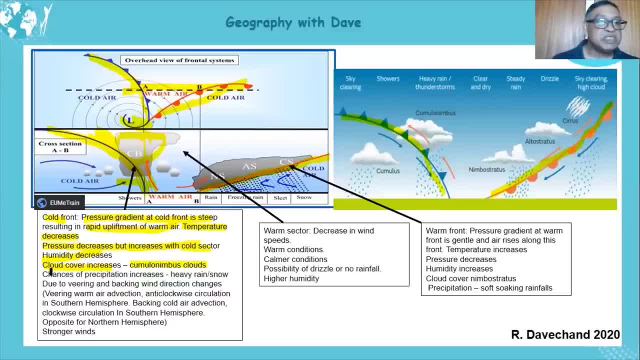 of vertical extent, chances of precipitation increases. it can be heavy rainfall, snow. that may happen all right over these areas. all right, so precipitation increase, you can get heavy rainfall. we'll do a case study later. you'll see that. all right, it can be heavy rainfall, snow happening. 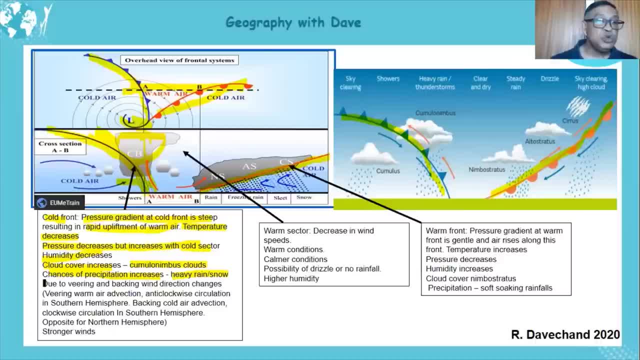 etc. all right, even due to veering and backing. wind direction changes- all right. veering and backing. now what is that? okay? uh? veering is when warm air- all right. uh, due to eviction, all right. actually has a change and it turns anti-clockwise, all right. 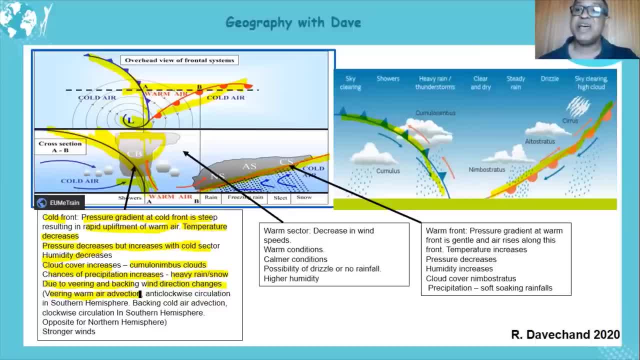 in the southern hemisphere. as it rises it turns anti-clockwise in the atmosphere. that is veering, all right anti-clockwise. and in the southern hemisphere and backing when cold air advection takes place, there is a clockwise circulation in the southern hemisphere, so veering changes. 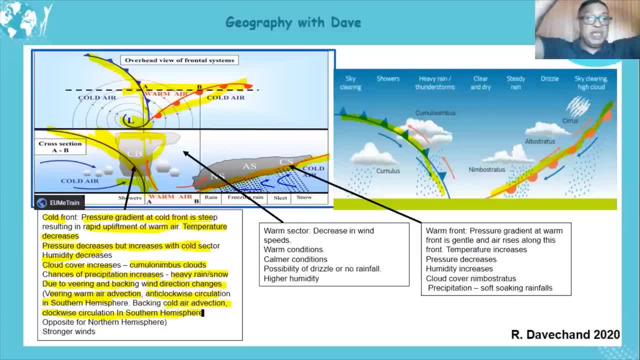 all right in the northern hemisphere. all right, anti-clockwise, as the warm air advection occurs when the liquid moves in the atmosphere horizontally. you understand, you get it anti-clockwise and with the cold air advection you have a clockwise circulation. now these changes actually change. 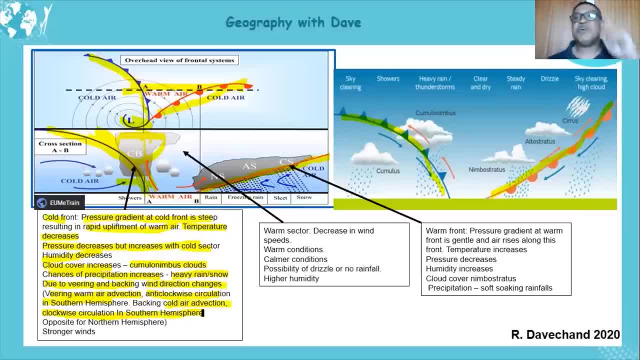 the direction of the movement of the air. all right, of course. the opposite is in the northern hemisphere, All right. Northern hemisphere has the opposite: Veering is clockwise, Backing is anticlockwise in the northern hemisphere. And because of these movements, the winds get stronger. All right, Stronger Because directions are changing at times and the winds get stronger. 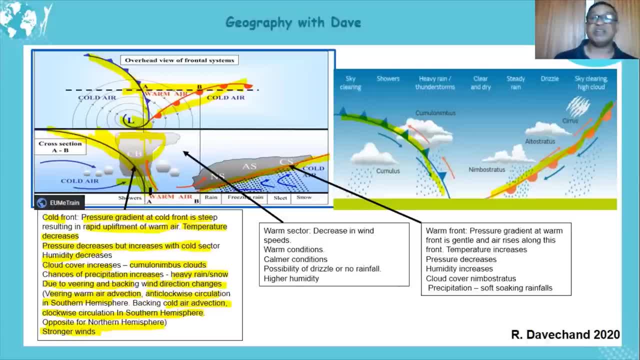 That is basically cold front situations. In the warm sector there's decrease in wind speeds, All right, Because it's warm. There's not much upliftment happening here until the cold front comes in, You understand. So it's just warm conditions, And if it's warm there's not much upliftment. Wind speeds are low. 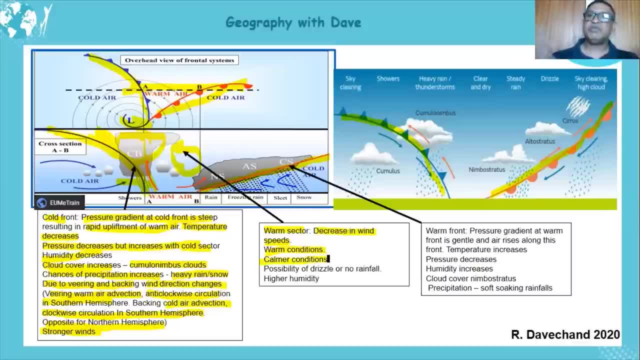 All right, Calmer conditions because wind speeds are low. Therefore it'll be calmer conditions, But it's not moving. Possibility of some drizzle If there's a little condensation. But sometimes we have no rainfall here And the higher humidity here because the air is moist, There's not much condensation, So the humidity is higher. 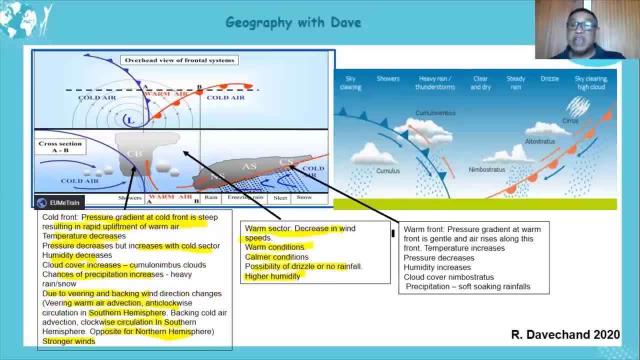 Can you see what I'm doing to this? I'm making sense of it. Let's look at the warm front now And you see the warm front. The pressure gradient at the warm front is gentle And if you notice this steep pressure gradient here, Can you see it Like the bulldozer, as I always say. 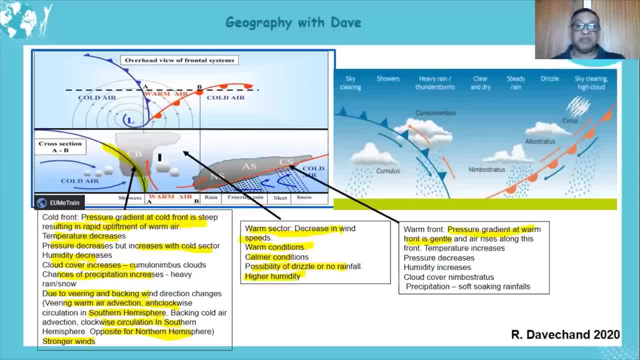 It's a steep pressure gradient. It's forcing rapid upliftment, But here it is gentle. You can see the gentle gradient here. So what happens here? Air rises along this front. Okay, It rises, All right. So as it's rises, obviously it's going to cool and cause some rainfall. So temperature increases because it is the warm front. 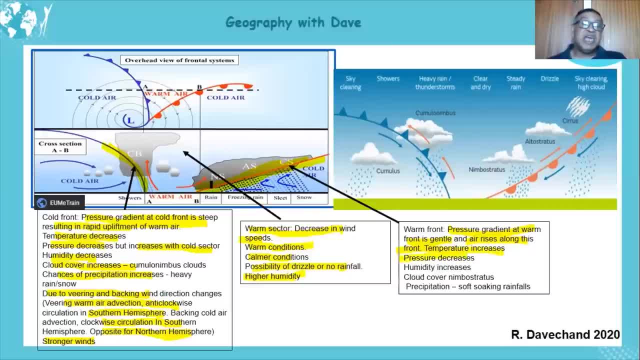 Pressure will decrease because air is rising. Therefore there's less air here, Not such a rapid movement, but still air is moving up. so pressure will decrease. humidity increases because as the air moves, all right, and then cloud cover occurs because as it moves up, you understand, it cools. 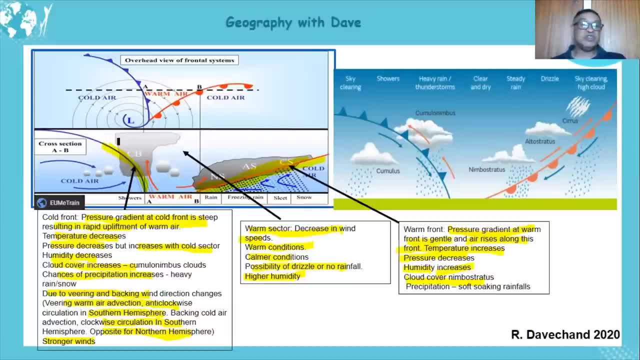 and condenses. but you're not going to get this huge cloud here. you're going to get more of a horizontal, i would say at an angle. you can't be totally horizontal, but you'll get a more one stretching out and that is your nimbo stratus clouds. right precipitation here is soft soaking. 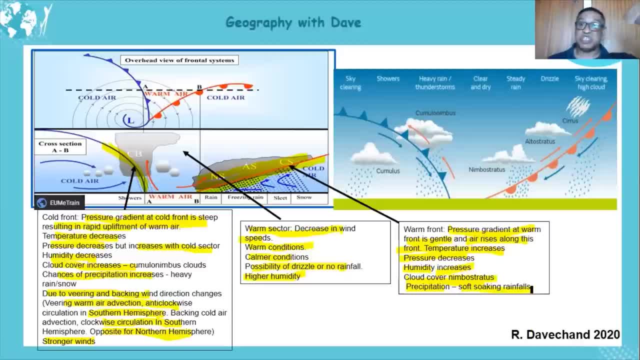 rainfalls different, say, from the cold front of the steep pressure gradient. rapid upliftment- yeah, the air rises along the warm front. so you've got different type of rainfall, everything you have reasons for, and it makes things simpler to understand. okay, i've got a little diagram here that shows you the different types of clouds. can you see it? 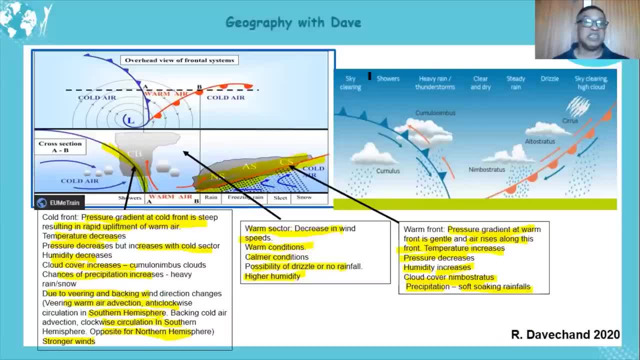 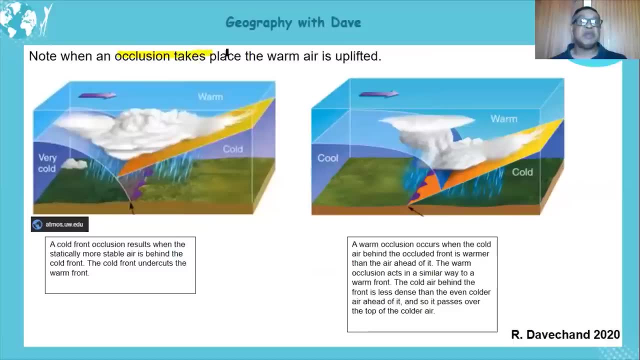 cumulonimbus here. this shows you a better vertical extent. it shows you the anvil shape, etc. okay, so that is your cross section and the weather stations, all right. now the occluded stage, and you know an occlusion takes place when warmer air is uplifted. i'd like to change that to. 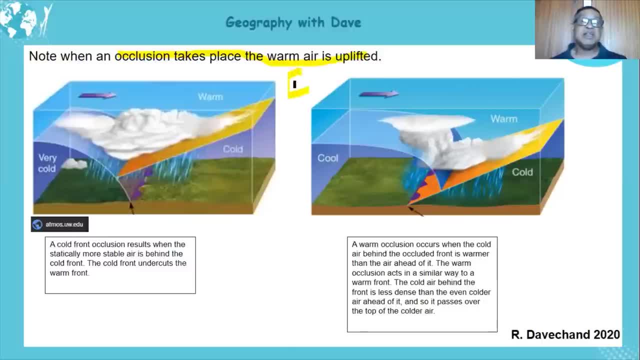 warm air. all right, warm air. i want to add that r? e r to here. warmer air, okay, so don't get a misconception. it's 20, some odd degrees, whatever. it can be much lower, but it is warmer than the other. a all right, warmer air is uplifted. that's an occlusion. all right, now let's look at we've got. 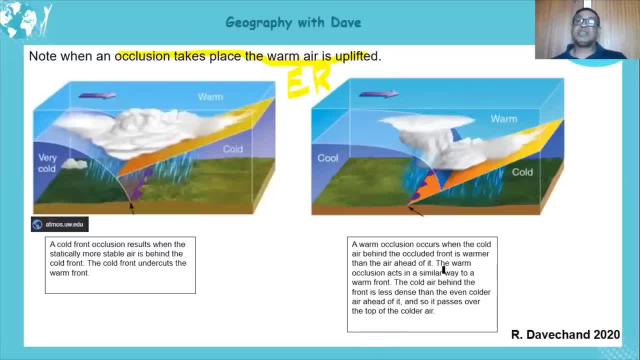 two types of occlusions: a cold front and a warm front occlusion. i learn as you. i don't know why you find the difficulty in this, but let's look at some simple things in identification. all right, you know, that's the cold front, that's the warm front, right. 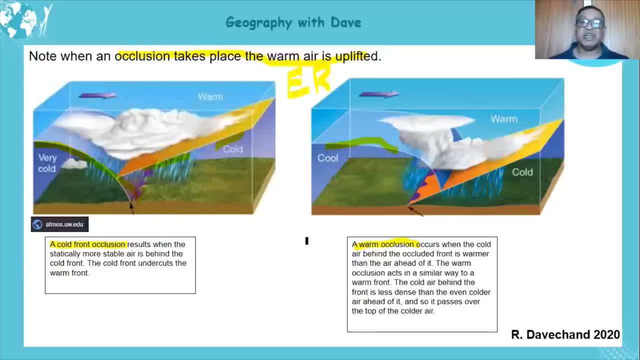 that's the cold front. that's the warm front here. okay, the warm front here. now, one way of identifying it is if it's a cold front occlusion. it seems like the cold front is touching the surface. can you see it? if it's a warm front occlusion, the warm front is touching the surface. 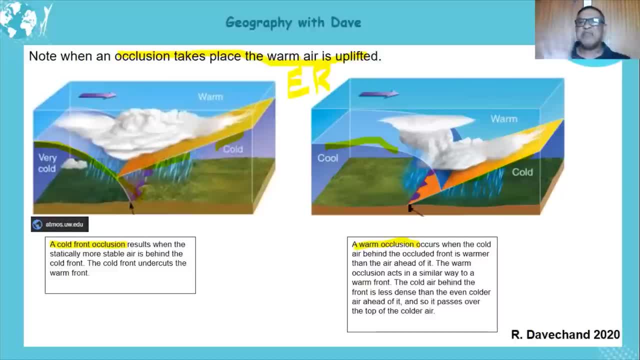 that's one thing that you can identify you, and if there, if any time, a question like that comes out, then you know: hey, cold front, warm front occlusion- all right. so warm front, cold front touching cold front occlusion. warm front touching warm front occlusion. right now, let's look a little bit more at this cold front occlusion results. 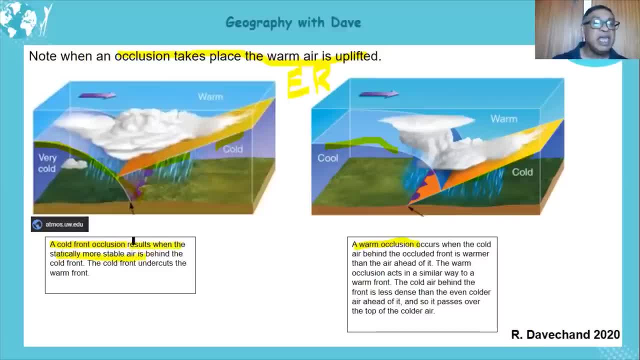 when the statically more stable a behind you understand the cold front, okay, uh. so this now, if you look at it there, all right, the cold front now undercuts the warm front, okay. so we say: is more stable, is colder, all right. when we say the statically more stable a, this means it's very cold, can you see it? and it's cold here, all right. so 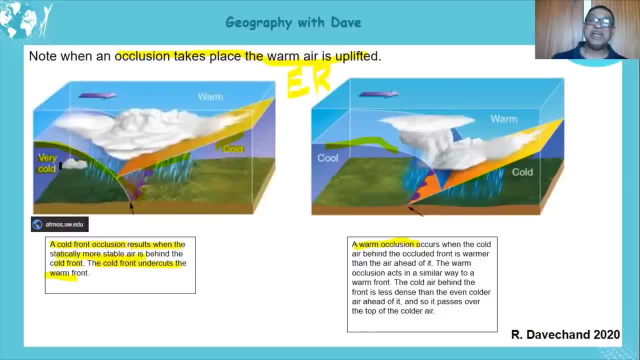 this area, literally, is warmer than that. okay, so what actually happens here is because this air is heavy, it's stable, a steep pressure gradient- okay, what it's going to do, it's going to go and undercut the warm front and as it goes through, it undercuts and pushes the air up. okay, in the 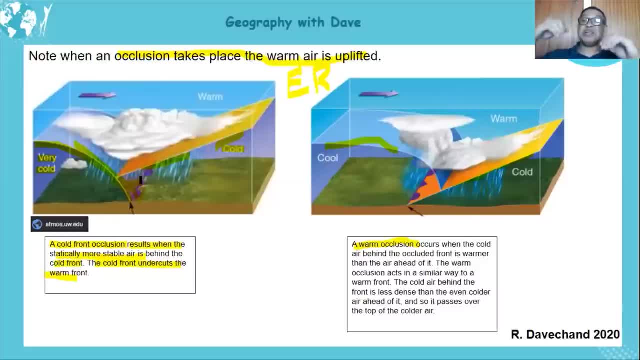 occlusion stage. that's a cold front occlusion- okay, cold air from cold front coming through, all right. so we say it's more stable, it's colder, it's forcing the warm air up, it's going underneath, undercutting and pushing it up. that is why it's touching the surface with the warm front occlusion. 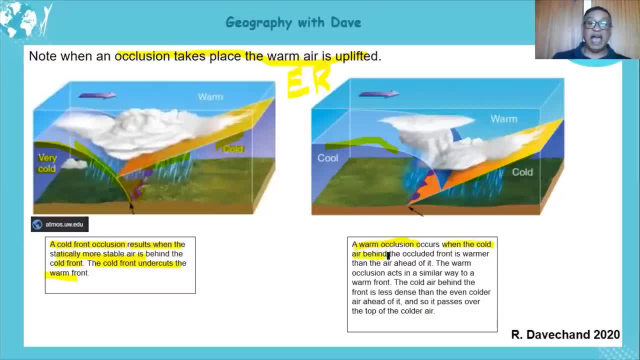 now watch this, when the cold air behind the occluded front is warmer, can you see it's cool here and it's cold here. can you see it? so behind there it's cooler and cold. so relatively, this air is warmer than this air. so what happens now? then the air ahead of it, can you see cold, cool. 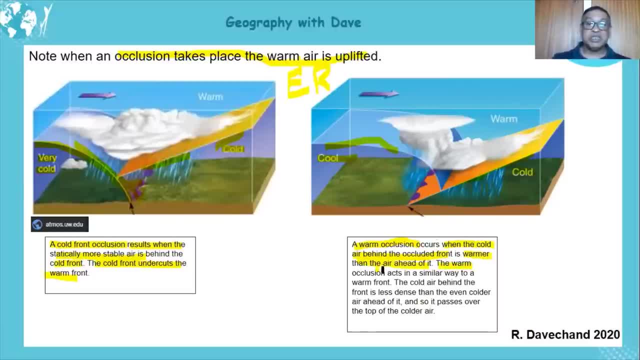 so what happens now in the warm occlusion acts in a similar way to a warm front. the cold air behind the front is less dense, can you see it? because it's cooler and that's cold, then even the colder air above it. it's colder here, so it passes over the colder air. 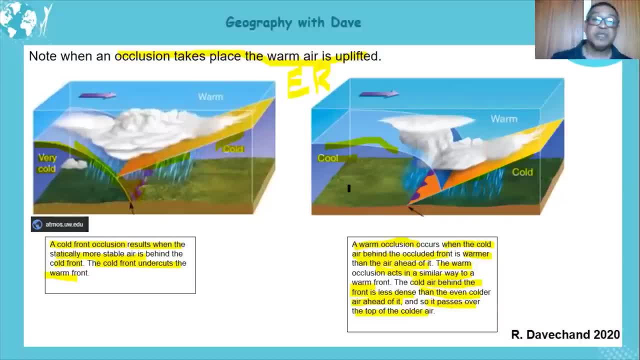 so because this is colder, it's more stable and this is cooler behind the occluded front. so what happens to this egg? it goes over the cold air and that is why the warm front touches the cold air, bringing water through from the air behind the occluded front, from around the inner halfway point. 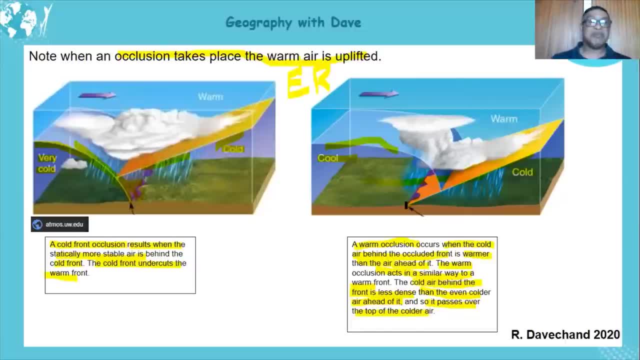 and it blows up. also a lot of the air produced by the cool front trusses, not because of the éx ролiphこと, all the of the air in it goes approximately directly to the cours of the occluded front and in thečt shortage these air make the success okay. so again, both cases, the so-called 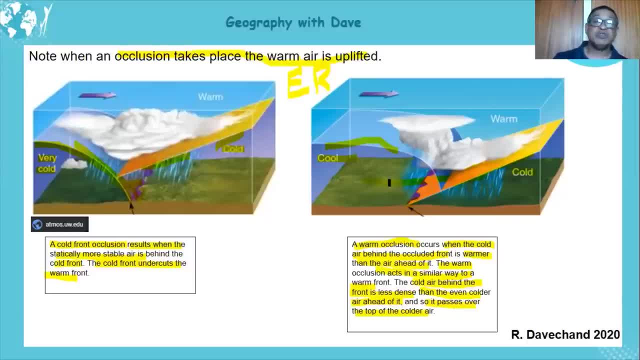 warmer air is pushed up. you understand, yeah, this is, the warmer air rises above, okay, it overrides the cold air, goes over, okay. i can understand. it's quite a complex thing, guys, but you remember those simple things. i've spent a little time on it. now remember that. 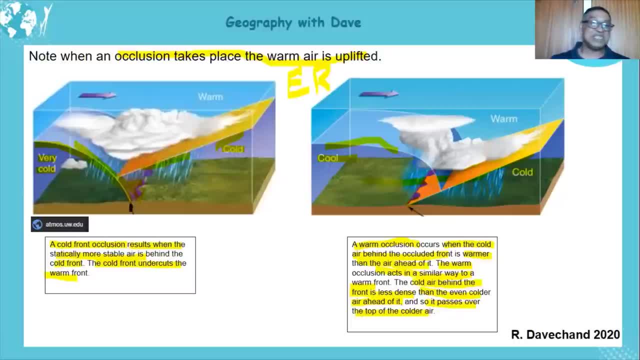 to identify alone. again, the cold front is touching the surface. cold front occlusion. the warm front is touching the surface. warm front occlusion. yeah, the air behind is colder, so it uplifts the air or undercuts the air in front of it of the warm front which has a higher 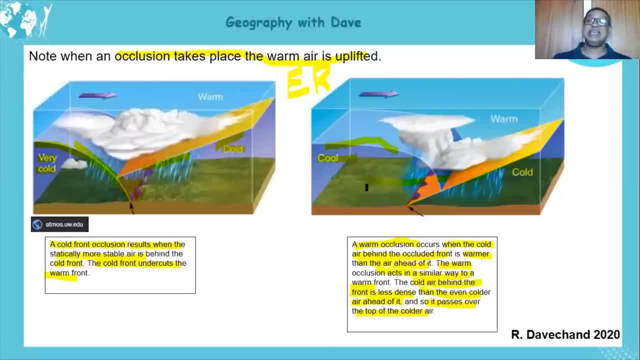 temperature: yeah, it's behind, the air is cooler and the air head is. uh, is cool and the air head is cold- lower temperature and therefore the cooler air overrides, it, goes over and rises. okay, i've spent a lot of time and your data on that. okay, right. 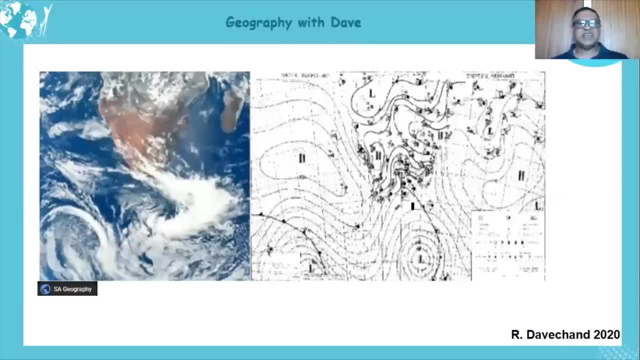 let's look at some synoptic interpretations, etc. now can you see here the dense cloud cover, learners? that is your cold front. you can see the cumulonimbus clouds- dense cloud cover, all right, that's your cold front hitting southern africa. yeah, can you see it? all right, there's. 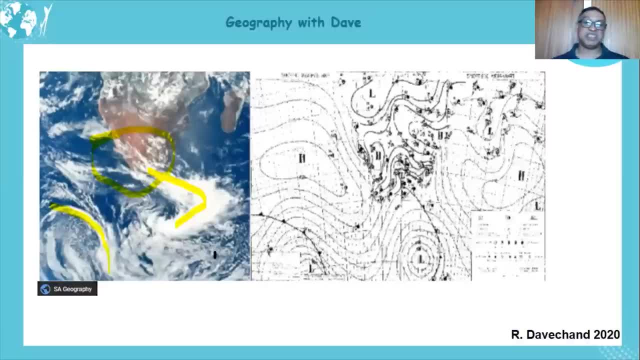 another one coming in down here. you can see that white patch, all right there. it is down here and this one has come through. can you see it here how the synoptic map is made? by looking at the satellite and you can clearly see the high pressures are in the northerly positions, can you? 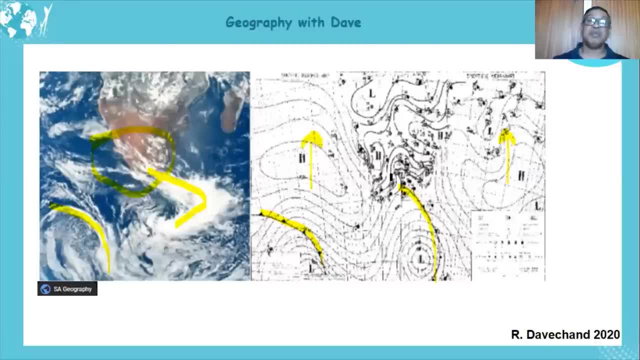 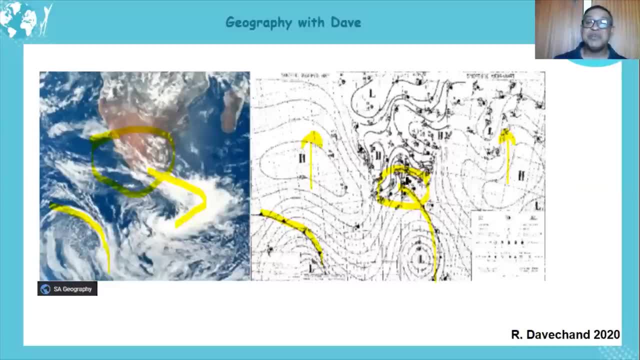 in color. in color. all right because it shows you cloud cover. all right because it shows you cloud cover. all right because it shows you cloud cover. cumulo numbers, clouds. can you see it? cumulo numbers, clouds. can you see it? cumulo numbers, clouds. can you see it? cumulo numbers, clouds, as it's moving. 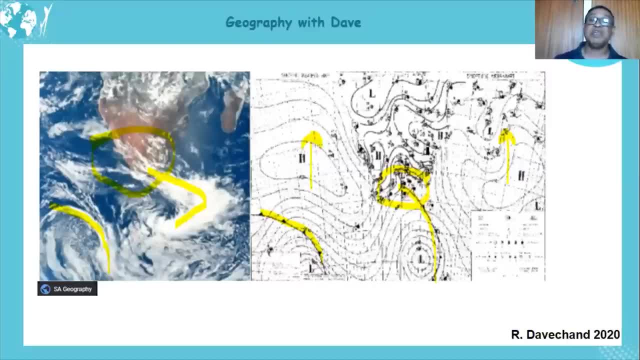 cumulo numbers: clouds as it's moving. cumulo numbers: clouds as it's moving. yeah, you may see some clear patches, i do. yeah, you may see some clear patches, i do. yeah, you may see some clear patches, i do apologize, not very clear. apologize, not very clear. 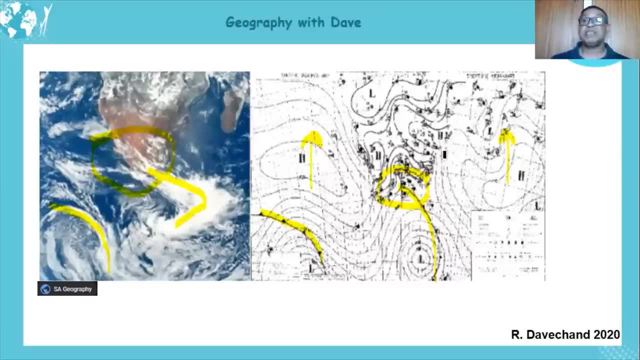 apologize, not very clear the the map itself, but you see some the the map itself, but you see some the the map itself, but you see some clearer patches, clearer patches, clearer patches, partially cloudy, etc. okay, because the cold partially cloudy, etc. okay, because the cold partially cloudy, etc. okay, because the cold front has not gone there yet. 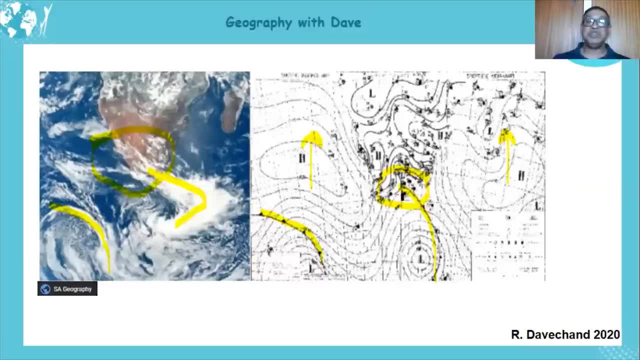 front has not gone there yet. front has not gone there yet. okay, say when where the symbols will show. okay, say when where the symbols will show. okay, say when where the symbols will show changing in wind speeds: greater wind. changing in wind speeds. greater wind. changing in wind speeds. greater wind speeds. 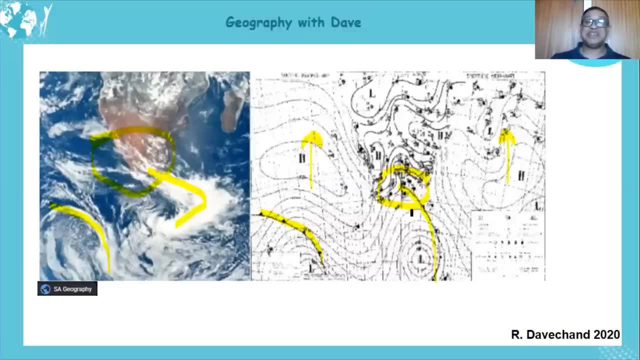 speeds: speeds- all right. overcast conditions: all right, overcast conditions, all right, overcast conditions, all right. so this is your summer northerly, all right. so this is your summer northerly, all right. so this is your summer northerly position. position, position, right. uh, it shows you another one here. 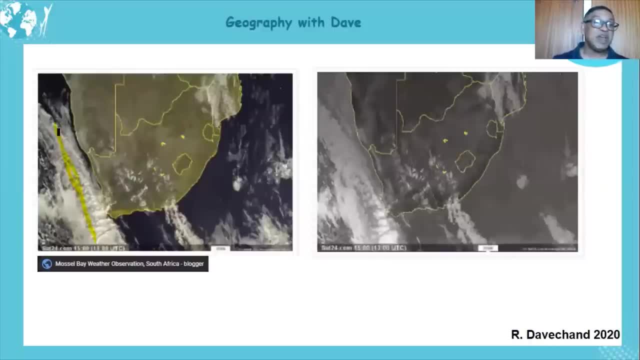 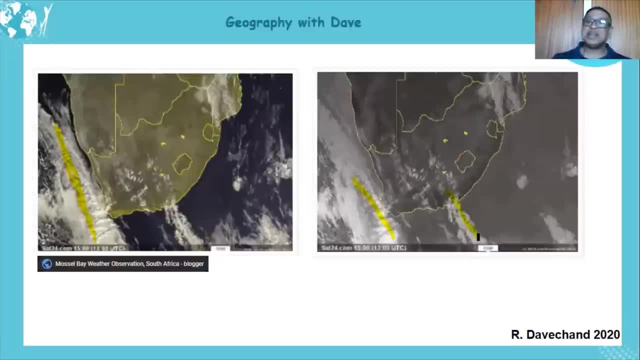 the band of clouds: yeah, cold front is now moved. the band of clouds- yeah, cold front is now moved over over over cold front. you understand brilliant if you cold front, you understand brilliant. if you cold front, you understand brilliant if you look at these satellite images from: look at these satellite images from: 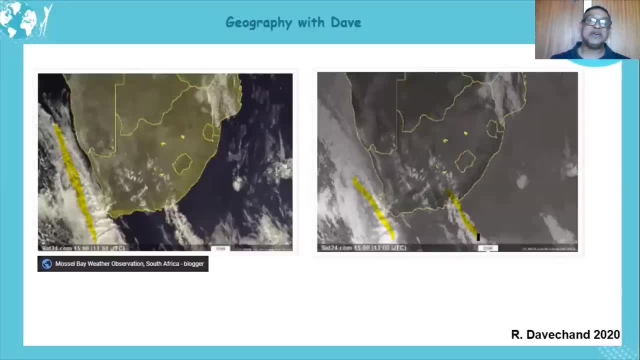 look at these satellite images from here. the synoptic map is here. the synoptic map is here. the synoptic map is made all right. i found this one made all right. i found this one made all right. i found this one very enjoyable. all right because this. 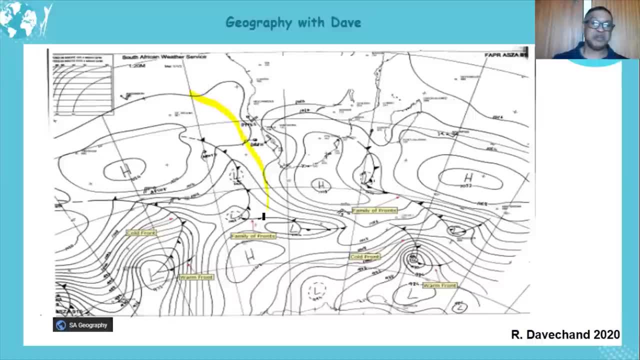 very enjoyable, all right, because this very enjoyable, all right, because this is the bugger, as i say, is the bugger as i say, is the bugger as i say. this one is the south atlantic high, is. this one is the south atlantic high is. 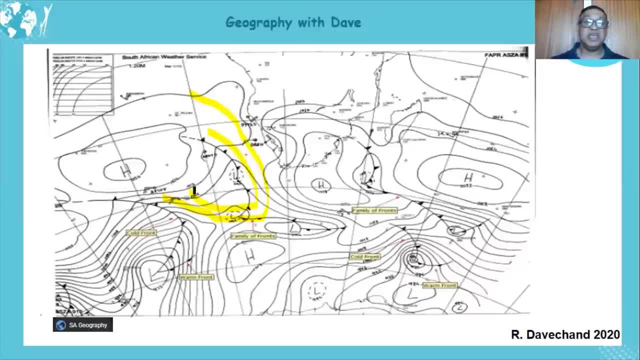 this one is the south atlantic high, is very strong and this is the one that very strong, and this is the one that very strong, and this is the one that ridges, ridges, ridges. okay, look at this one, this kalahari high. okay, look at this one, this kalahari high. 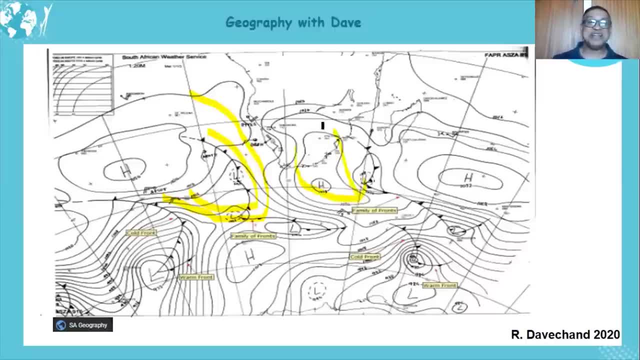 okay, look at this one. this kalahari high is doing some religion here, is doing some religion here, is doing some religion here, okay, so it's quite unusual that you see. okay, so it's quite unusual that you see. okay, so it's quite unusual that you see that. 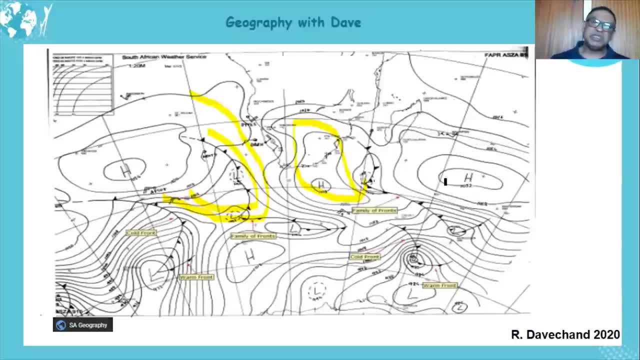 that that and it's blocking to a certain extent. and it's blocking to a certain extent. and it's blocking to a certain extent. you notice they're starting to move north. you notice they're starting to move north. you notice they're starting to move north. they're starting to move north learners. they're starting to move north learners. they're starting to move north learners to a certain extent. so if i had to look to a certain extent, so if i had to look to a certain extent, so if i had to look at the season of this, at the season of this, 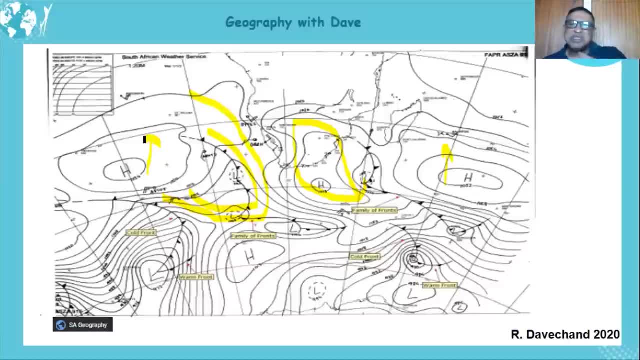 at the season of this. this higher order it's towards the latter. this higher order it's towards the latter. this higher order it's towards the latter part, part, part of your winter season. so they still of your winter season, so they still of your winter season, so they still uh, uh, it's starting to uh, sorry, your. 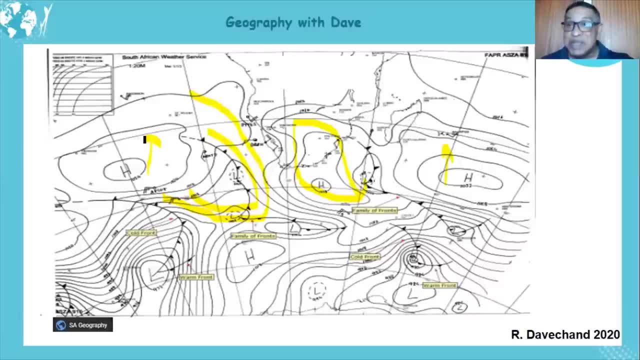 uh, uh, it's starting to uh sorry your. uh, uh, it's starting to uh sorry your. the winter season is moving towards your. the winter season is moving towards your. the winter season is moving towards your. summer season: all right, it's moving. summer season: all right, it's moving. 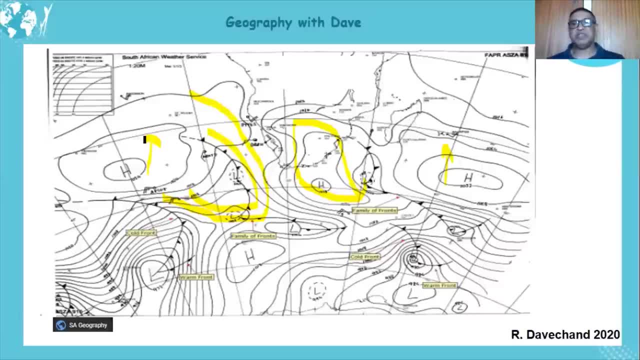 summer season. all right, it's moving towards your spring, towards your spring, towards your spring, and then your summer. i'm forgetting my and then your summer. i'm forgetting my and then your summer. i'm forgetting my seasons also, seasons also, seasons also. okay, so it's starting to move up, but 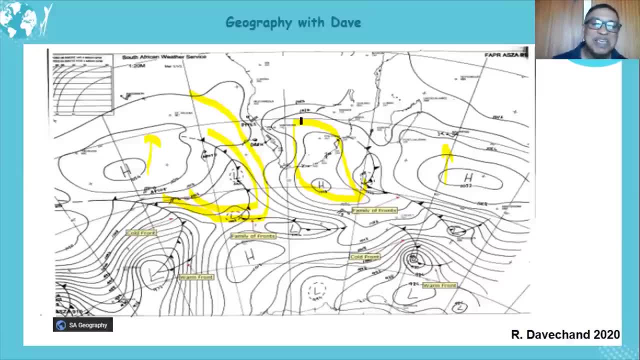 okay, so it's starting to move up. but okay, so it's starting to move up, but there's still some blocking. there's still some blocking, there's still some blocking. and i found this to be interesting, and i found this to be interesting and i found this to be interesting, how the kalahari high is doing some. 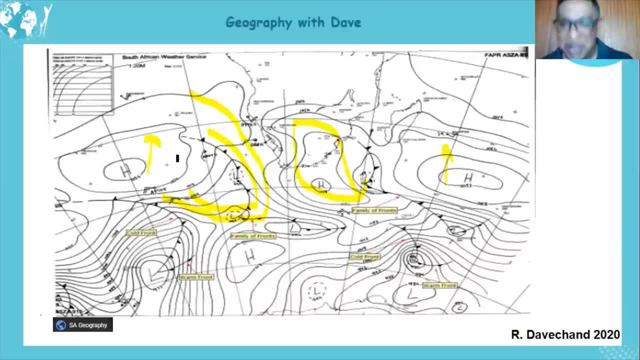 how the kalahari high is doing some, how the kalahari high is doing some blocking, blocking, blocking. mostly this one does the blocking of the. mostly this one does the blocking of the. mostly this one does the blocking of the when it ridges, of the cold fronts. 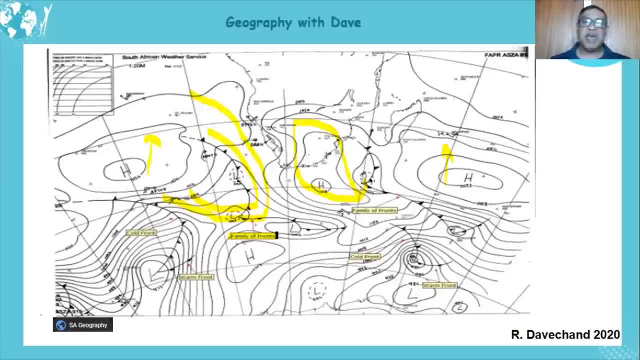 when it ridges of the cold fronts. when it ridges of the cold fronts, okay, and you look at the word here. okay, and you look at the word here: okay, and you look at the word here: learners, learners, learners. family of fronts. when there's a few. 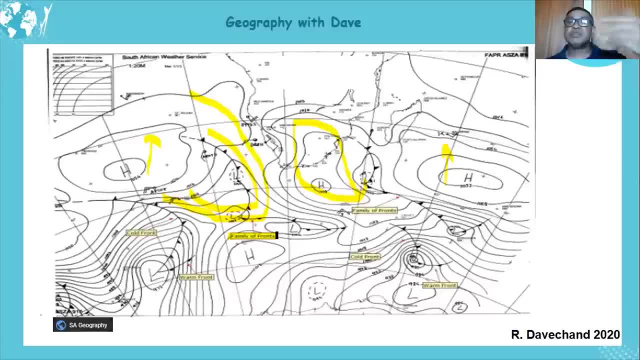 family of fronts when there's a few, family of fronts when there's a few. uh, uh, uh, uh. with latitude cyclones coming in, we call. with latitude cyclones coming in, we call: with latitude cyclones coming in, we call it a family. it a family. it a family of mid-latitude cyclones. so i'm going. 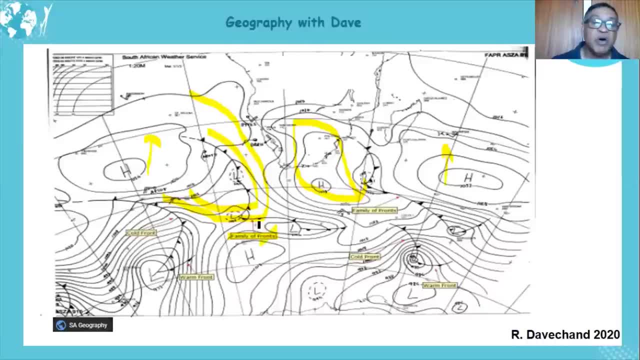 of mid-latitude cyclones. so i'm going of mid-latitude cyclones, so i'm going to change this word, to change this word, to change this word: front sample across and call it front sample across. and call it front sample across and call it family of mid-latitude cyclones. 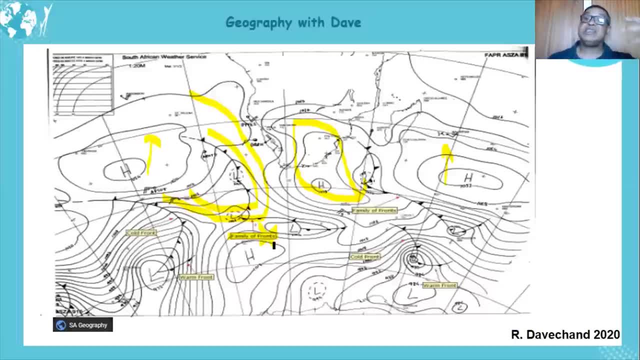 family of mid-latitude cyclones. family of mid-latitude cyclones. when there's fuel like there's three, when there's fuel like there's three, when there's fuel like there's three. mid-latitude cyclones. mid-latitude cyclones. mid-latitude cyclones. it is a family of middle latitude. 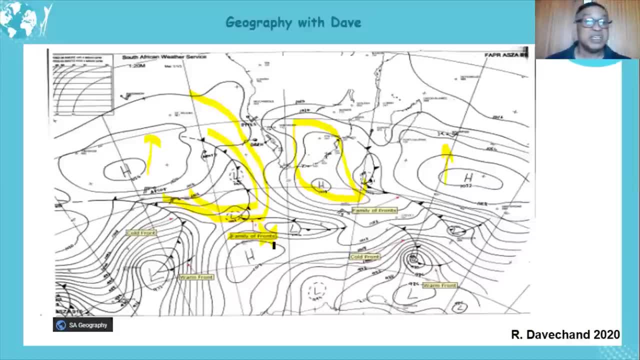 it is a family of middle latitude. it is a family of middle latitude. cyclones that's occurring, cyclones. that's occurring cyclones that's occurring. a few like three occurring in the area. a few like three occurring in the area. a few like three occurring in the area. look at this a beautiful. 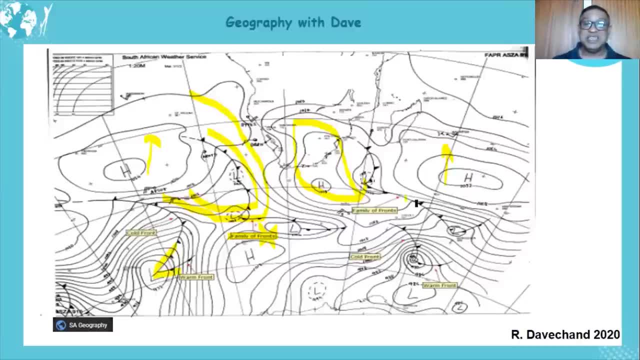 look at this, a beautiful. look at this, a beautiful occlusion is starting here. can you see? occlusion is starting here. can you see? occlusion is starting here. can you see? this is in the mature stage. this is in the mature stage. this is in the mature stage of this area. all right, 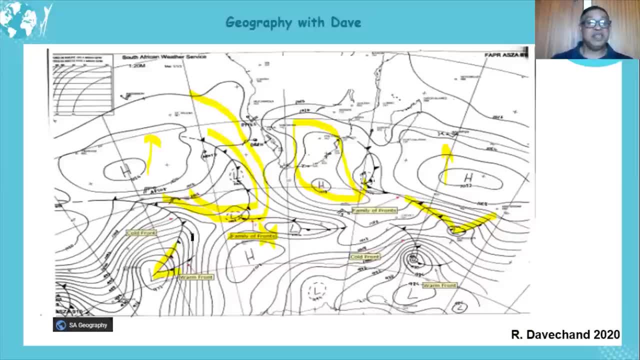 of this area, all right, of this area, all right, although this is older, although this is older, although this is older than this. why is it older than this, than this? why is it older than this than this? why is it older than this? because it moves from west to east. 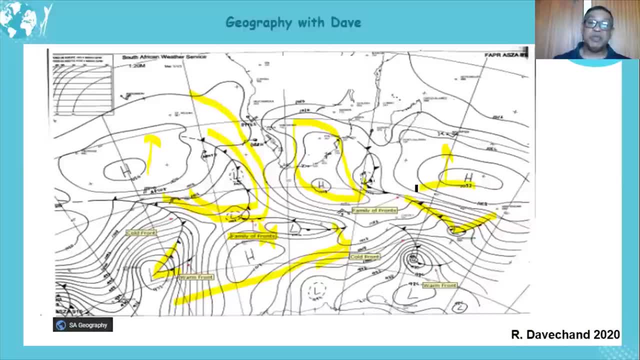 because it moves from west to east. because it moves from west to east. you understand, therefore, this one, will you understand, therefore, this one will you understand. therefore, this one will be, be be older than this one that we have here, older than this one that we have here. 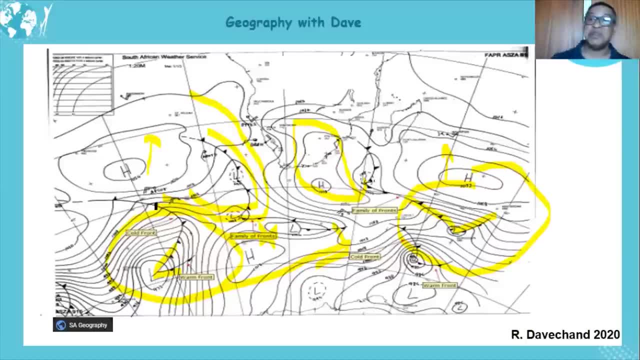 older than this one that we have here. okay, that's also working out which one. okay, that's also working out which one. okay, that's also working out which one is older and which one is newer is older, and which one is newer is older and which one is newer west to east. okay, some interesting stuff. 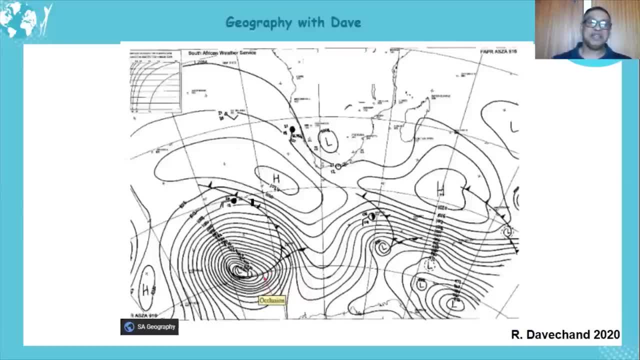 west to east. okay, some interesting stuff west to east. okay, some interesting stuff there, there, there. ah, we can see a nice one here, all right. ah, we can see a nice one here, all right. ah, we can see a nice one here, all right, it's a beautiful one here. and what is? 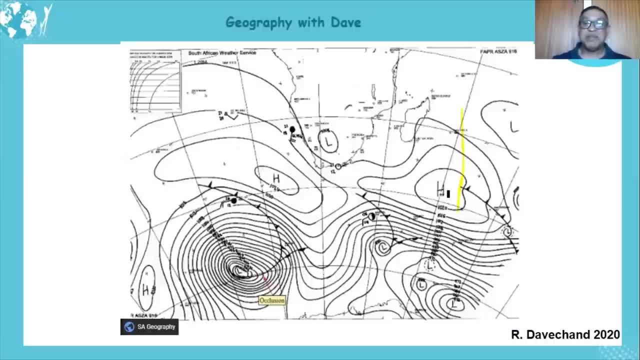 it's a beautiful one here. and what is? it's a beautiful one here. and what is this? this, this, clearly, you notice your high pressure. clearly, you notice your high pressure. clearly, you notice your high pressure. systems, systems, systems are in the southerly position, are in the southerly position. 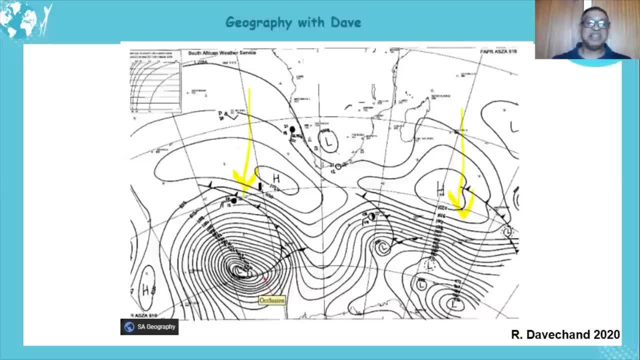 are in the southerly position. all right, so it's more summer conditions. all right, so it's more summer conditions. all right, so it's more summer conditions. hey, hey, hey. and it's. can you see the ridging this? and it's, can you see the ridging this? 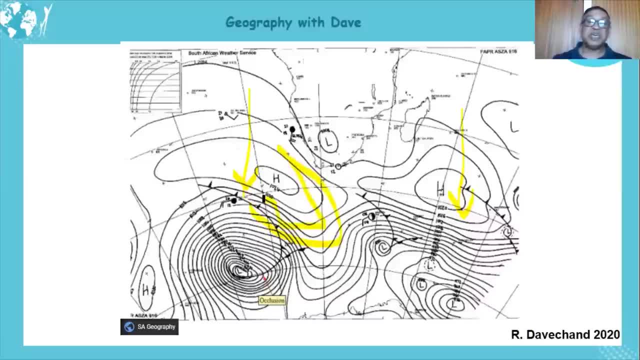 and it's. can you see the ridging? this one does the most. one does the most. one does the most. it ridges okay and blocks the gold. it ridges okay and blocks the gold. it ridges okay and blocks the gold fronts from affecting the country. it's. 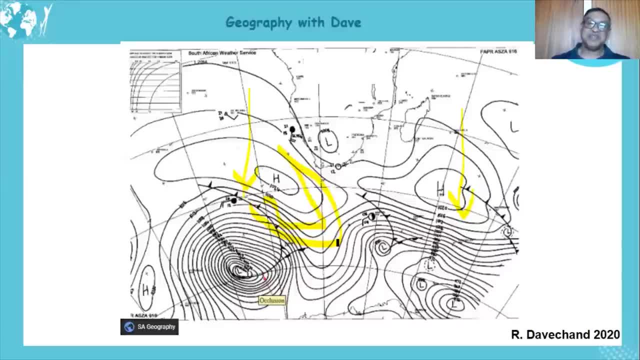 fronts from affecting the country. it's fronts from affecting the country. it's going to push it further, going to push it further, going to push it further south. okay so, typical sort of south. okay so, typical sort of south. okay so, typical sort of- uh, summer conditions. even this one, we 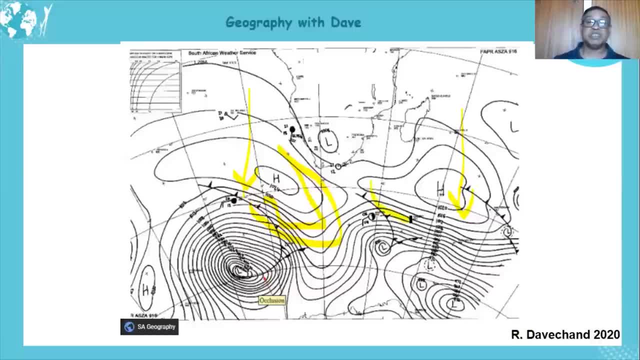 uh, summer conditions, even this one. we uh summer conditions, even this one. we don't mustn't forget about this one, don't mustn't forget about this one, don't mustn't forget about this one. he's also doing some reaching the south. he's also doing some reaching the south. 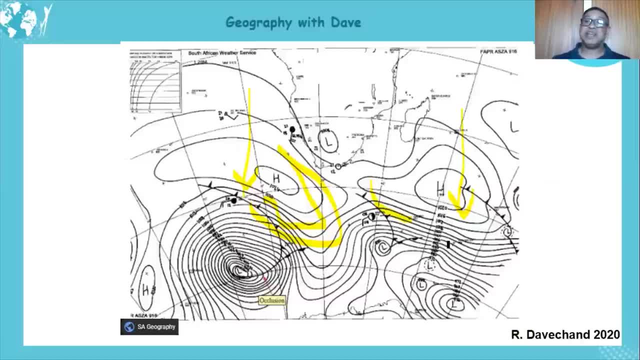 he's also doing some reaching the south indian high, indian high, indian high, and blocking it from coming in all right and blocking it from coming in all right, and blocking it from coming in all right. so these are some diagonal, so these are some diagonal, so these are some diagonal things. and if you look at these summer, 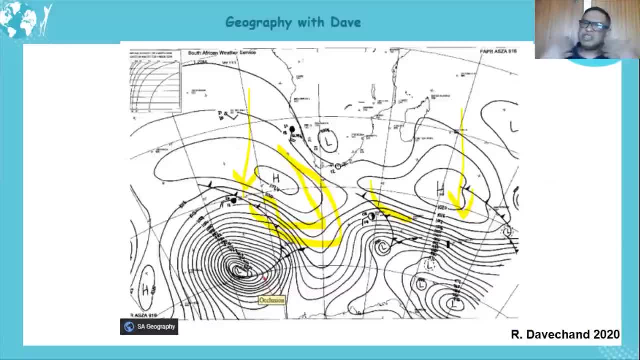 things. and if you look at these summer things and if you look at these summer, winter conditions, winter conditions, winter conditions, then you get a brilliant idea on a. then you get a brilliant idea on a. then you get a brilliant idea on a synoptic map- how it looks. 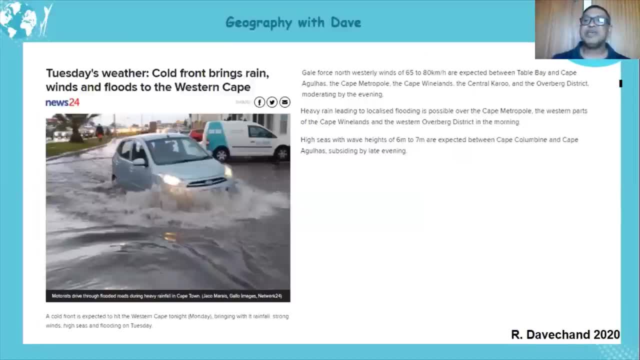 synoptic map: how it looks. synoptic map: how it looks okay. and then, lastly, i want to look at: okay, and then, lastly, i want to look at okay. and then, lastly, i want to look at this, this, this, okay, i'm not trying to make my face big. 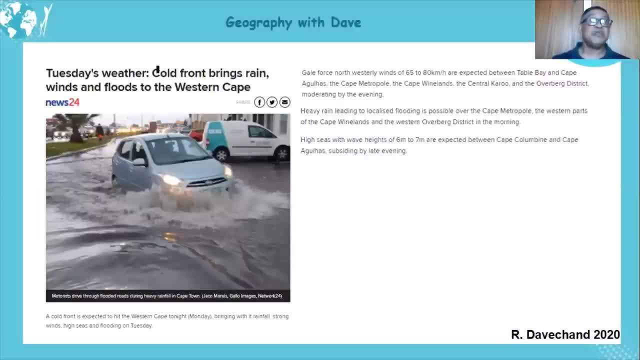 okay, i'm not trying to make my face big. okay, i'm not trying to make my face big, i'm not that important. i'm not that important. i'm not that important. look at, the cold front brings rain. and look at, the cold front brings rain and. 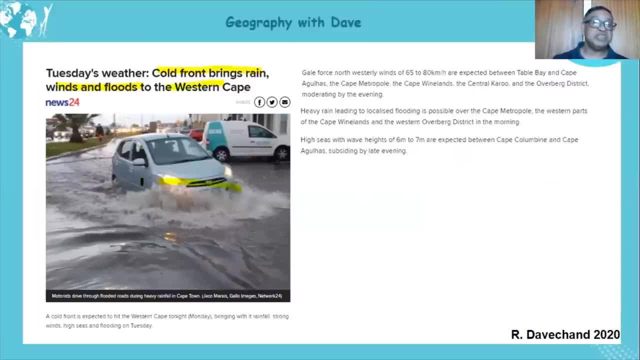 look at, the cold front brings rain and winds, winds, winds and floods to the western cape, you can, and floods to the western cape, you can. and floods to the western cape, you can see it here, the amount of water. see it here, the amount of water. see it here the amount of water. gale force, northwesterly winds. 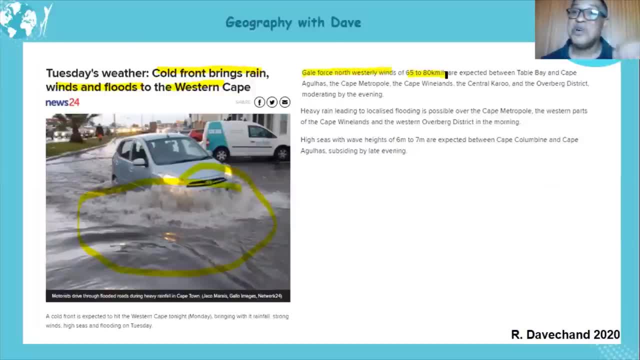 gale force- northwesterly winds. gale force- northwesterly winds of 65 to 80 kilometers. so it can bring of 65 to 80 kilometers. so it can bring of 65 to 80 kilometers, so it can bring strong winds. 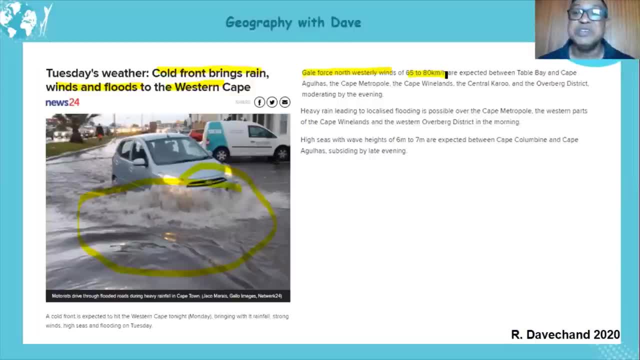 strong winds, strong winds that backing and fearing changing the that backing and fearing changing the that backing and fearing changing the direction of the winds. direction of the winds, direction of the winds. all right, i expected. between table bay. all right, i expected between table bay. all right, i expected between table bay and cape agalas and the cape metropolis. 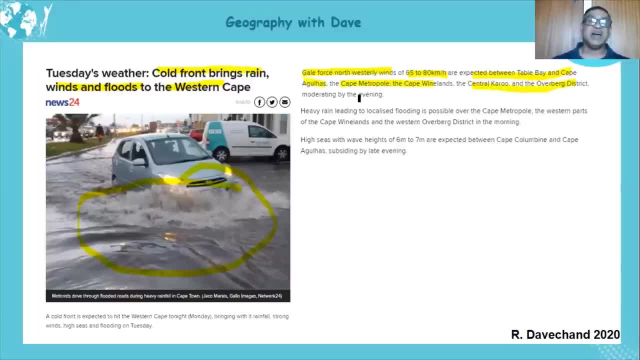 and cape agalas and the cape metapolis and cape agalas and the cape metropolis and winelands central karu- see the area. and winelands central karu- see the area. and winelands central karu- see the area that it covers. 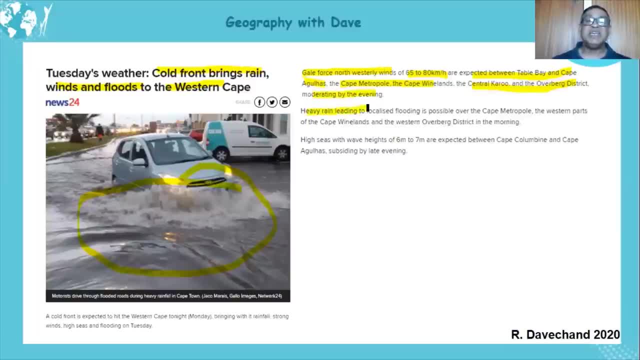 that it covers. that it covers moderating in the evening. cooling off. moderating in the evening: cooling off. moderating in the evening. cooling off heavy rains leading to localized flooding. heavy rains leading to localized flooding. heavy rains leading to localized flooding is possible over the cape metropole. 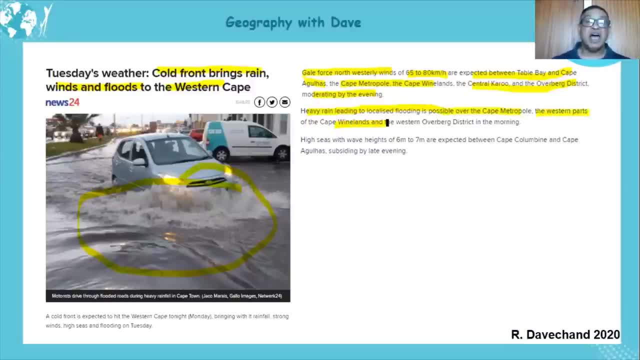 is possible over the cape metropole, is possible over the cape metropole, the western parts of the cape winelands, the western parts of the cape winelands, the western parts of the cape winelands, large areas. look at this high seas with. 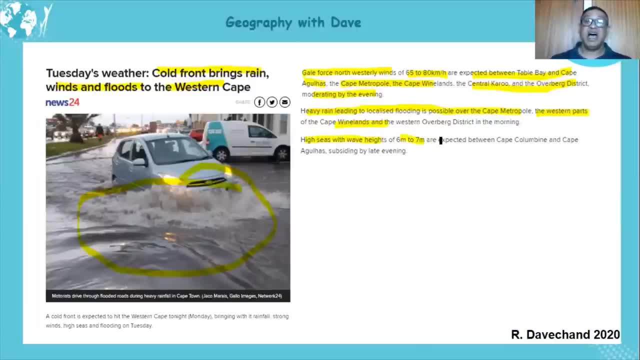 large areas. look at this. high seas with large areas. look at this. high seas with wave heights of wave heights of wave heights of six to seven meters are expected. between six to seven meters are expected. between six to seven meters are expected between it can destroy, whether it's the 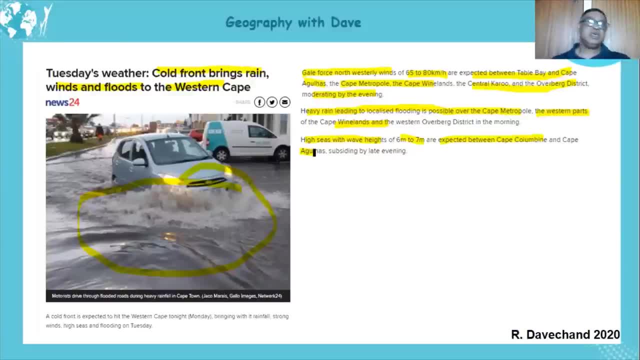 it can destroy, whether it's the, it can destroy, whether it's the farming road networks, farming road networks, farming road networks, people's homes, especially living in people's homes, especially living in people's homes, especially living in informal settlements, informal settlements, informal settlements damaging the natural environment. so we 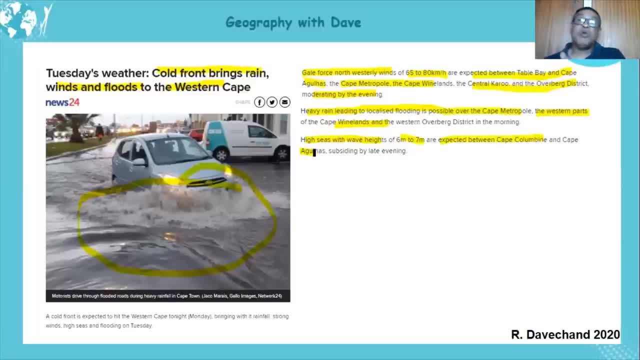 damaging the natural environment. so we damaging the natural environment. so we can do a lot of things, can do a lot of things. can do a lot of things and damage, but must also remember and damage, but must also remember and damage, but must also remember that sometimes it brings good rains. so 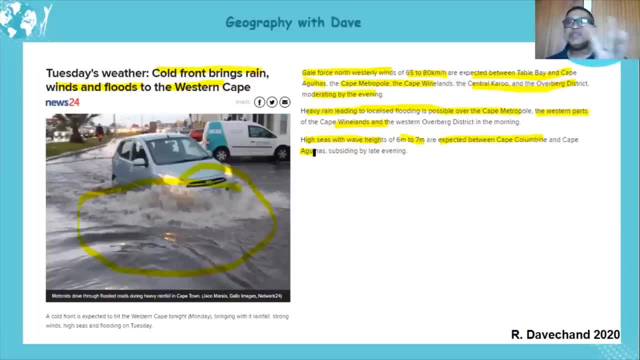 that sometimes it brings good rains, so that sometimes it brings good rains, so it can have a positive effect. it can have a positive effect. it can have a positive effect. you understand it brings in good rains. you understand it brings in good rains. you understand it brings in good rains which allow for crops to grow natural. 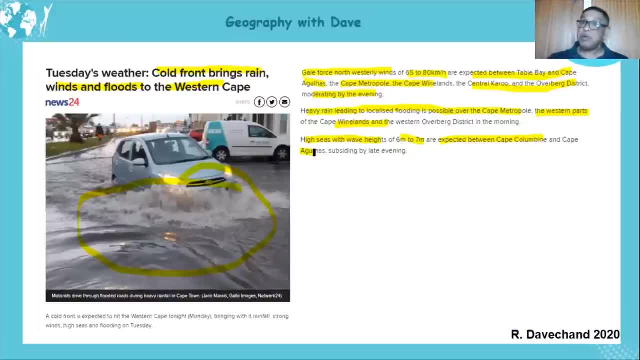 which allow for crops to grow natural, which allow for crops to grow natural, vegetation, vegetation, vegetation, water supply. so it can be positive water supply. so it can be positive water supply, so it can be positive, depending on the intensity, depending on the intensity, depending on the intensity of the rainfall and winds, etc. 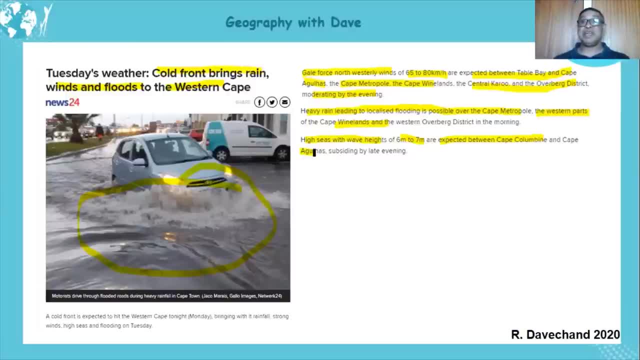 of the rainfall and winds, etc. of the rainfall and winds, etc. so it can be positive, even your snow. so it can be positive, even your snow, so it can be positive. even your snow, you understand, can be positive. people you understand can be positive. people you understand, can be positive. people love to see snow. 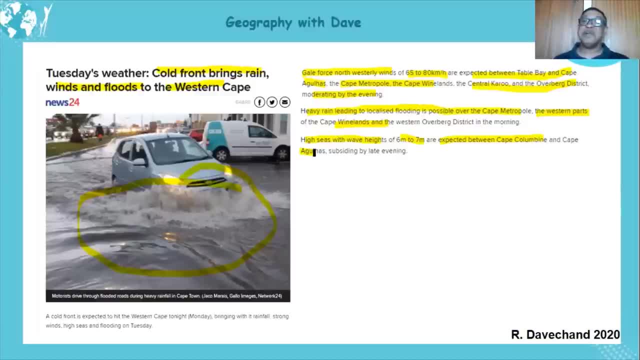 love to see snow. love to see snow, tourism, etc. which is brilliant for tourism, etc. which is brilliant for tourism, etc. which is brilliant for the economy of the area. all right, the the economy of the area. all right, the farming of the area. so it can have a positive or negative effect. learners, i hope you enjoyed. 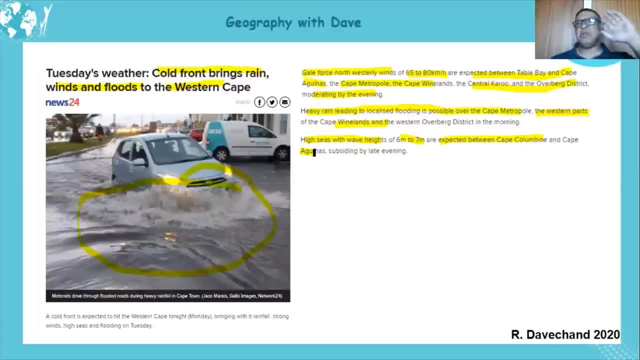 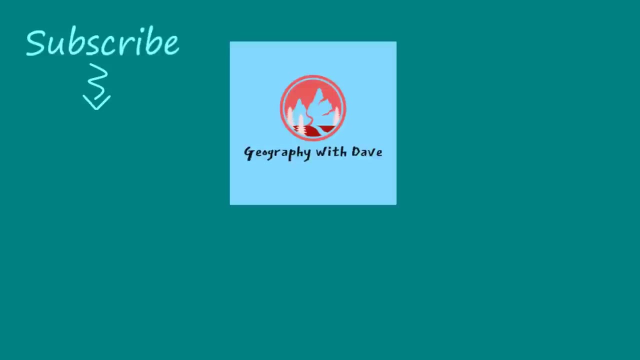 the lesson. i'm not putting any questions here. you've got loads of past papers. i've done some revision lessons also on youtube which you can refer to, so i hope you enjoyed it all the best. goodbye.